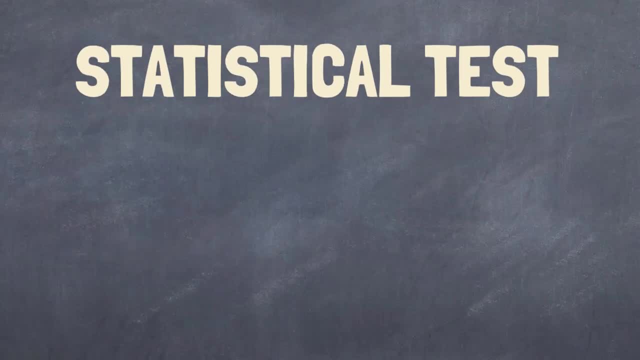 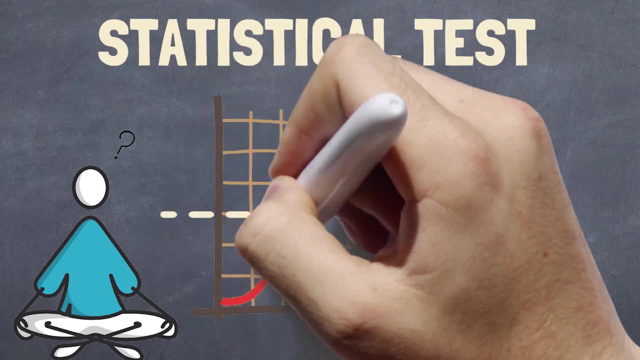 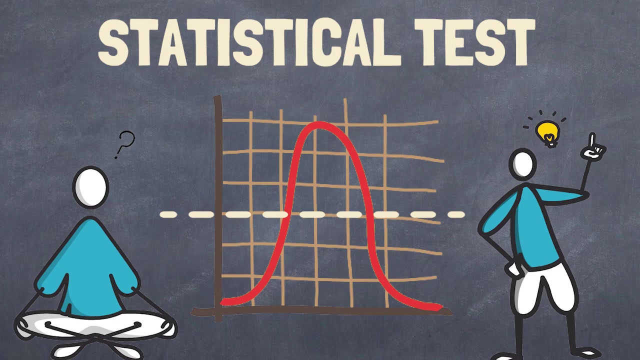 Welcome back to this Global Health YouTube channel. In this video, we're going to be talking about statistical tests: Which test to do when It's not complicated, and the key is to understand what question it is that you're asking. and when you understand the question, it becomes very easy to understand and interpret the results and to decide which tests to do when. So don't go away, stick with me, you're going to love this. 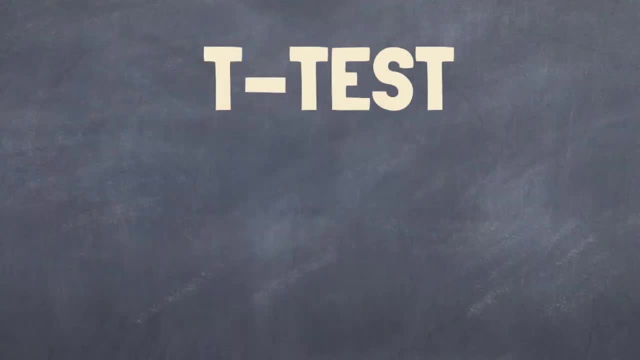 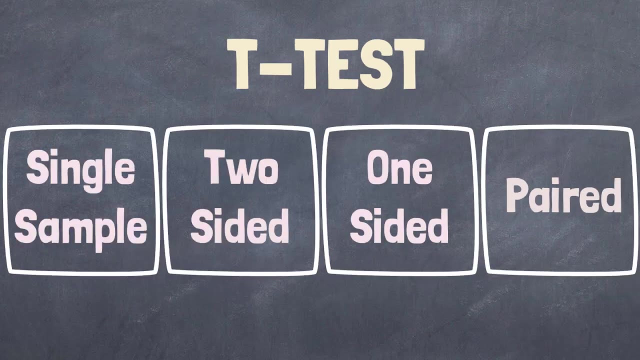 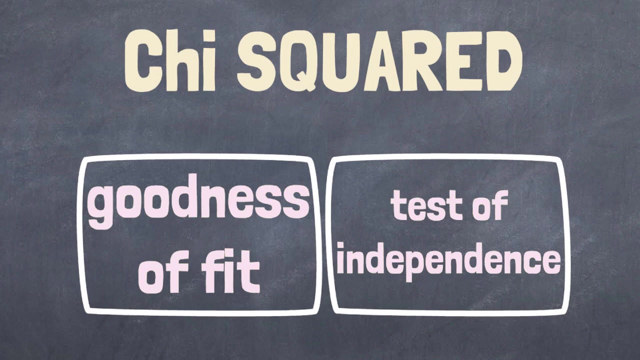 We're going to cover three things in this video: The t-test, ANOVA, which is analysis of variance, and the chi-squared test. For the t-test, there will be the single sample. there's going to be two-tailed, one-tailed and paired. We're going to do all four of those things. And for the chi-squared, there's the goodness of fit and, of course, there's also the test of independence. You're going to find all of this super duper easy to understand. so stick with me, don't go away. let's do this. 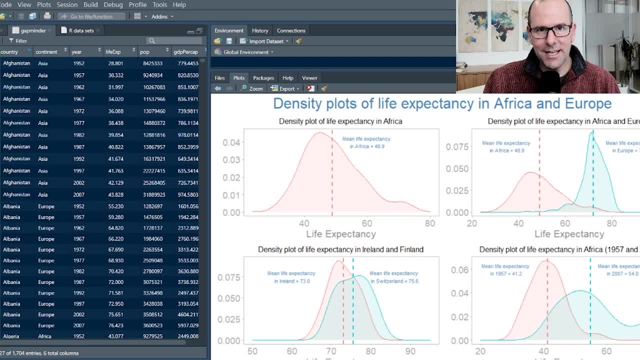 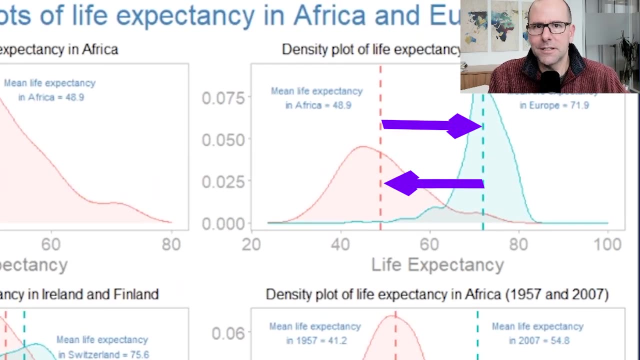 Let's talk about the t-test. I've got real data and real examples here and we're going to look at four different scenarios, four different applications. When we do a t-test, we're asking a question about the difference in means or averages- difference between two populations, or difference between one population at different points in time, or the difference in an average mean that we're seeing compared to some sort of hypothesized or presumed average, right or presumed mean. 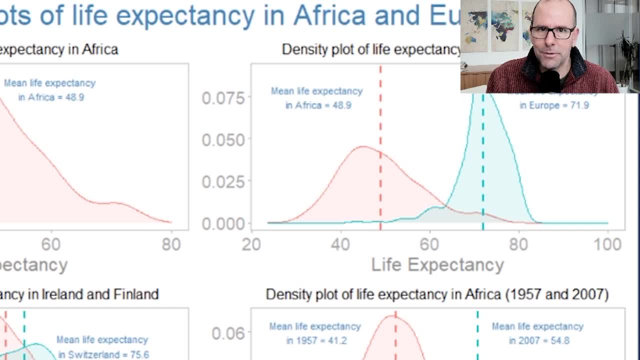 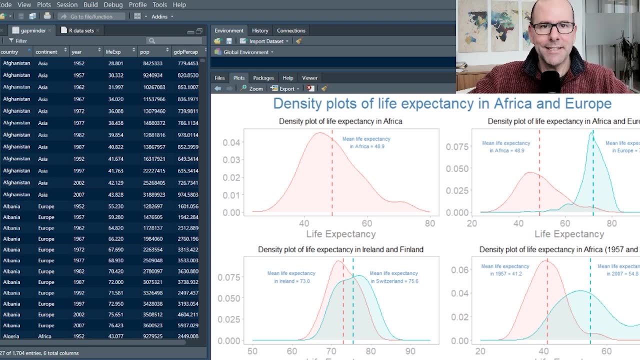 And we're asking the question: can from our sample data, can we make inference about the wider population? Is this somehow representative of the truth that's out there, Representative of the population from which the sample was taken? In other words, is this statistically significant? 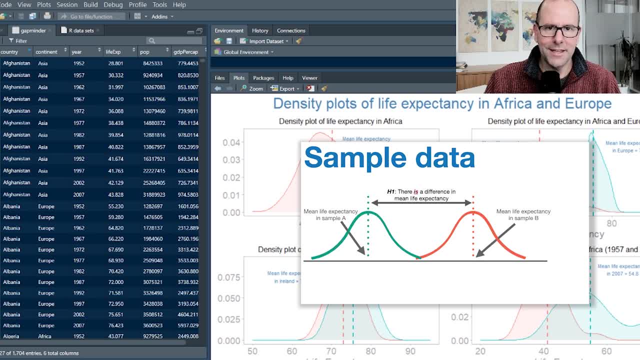 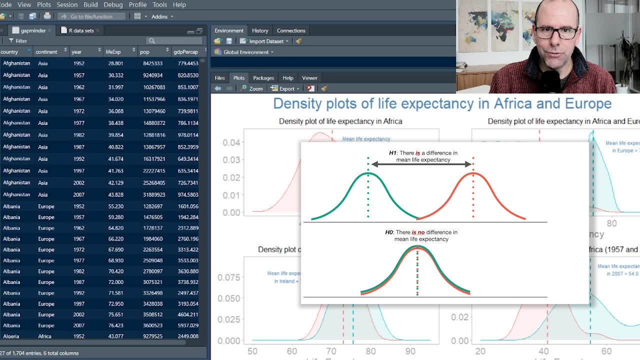 And this is how hypothesis testing works. We assume the opposite, the counterfactual, the antithesis. We assume that there's no difference in means between these two populations. If that were true, and we call that the null hypothesis. if that were true. 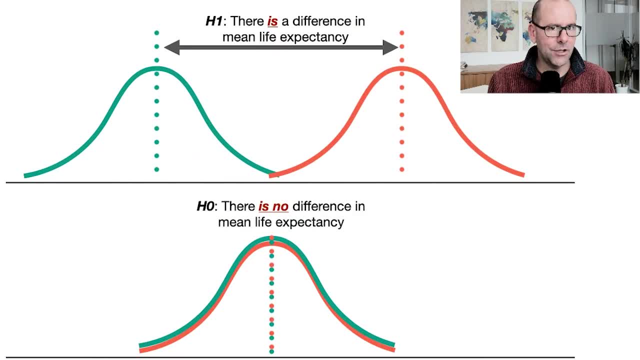 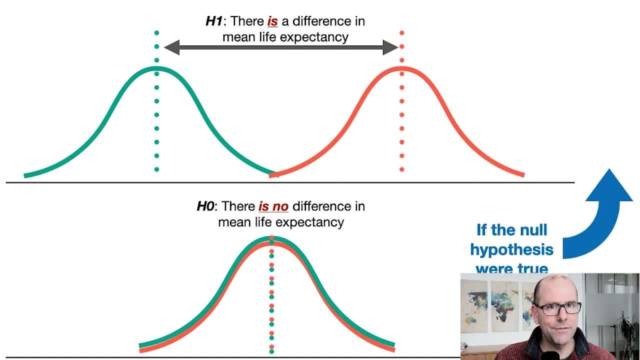 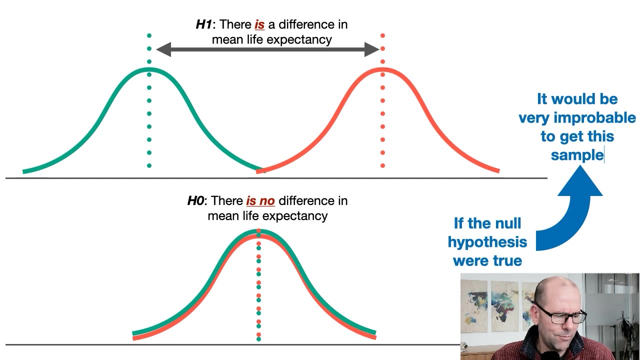 then how likely would it be that we would get a sample from the population that shows a difference that we're seeing or greater? What is the probability of that? If we find that that is very improbable- and we decide up front, by the way, we decide up front what we consider, what the threshold for what we would consider to be very improbable, what we mean by very- and we often use 5% if it's 5% or less in terms of likelihood or probability- if it would be very improbable to get a sample like we've gotten, if the null hypothesis were true. 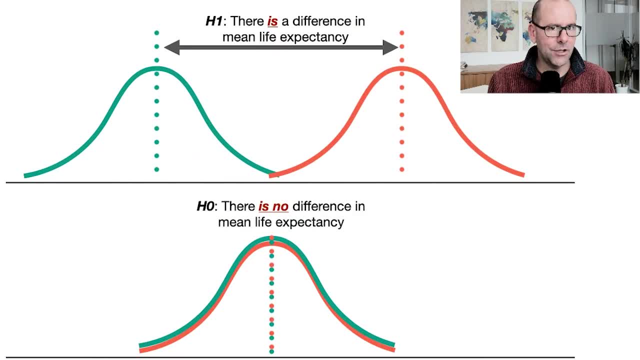 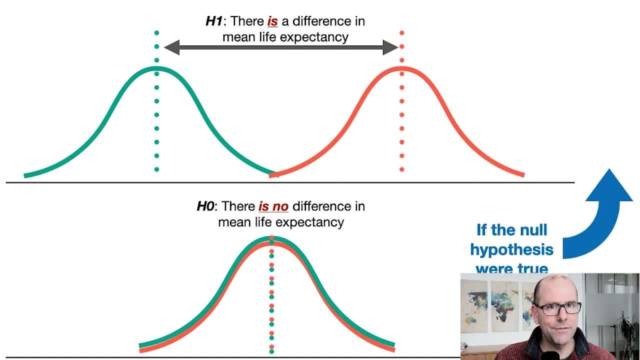 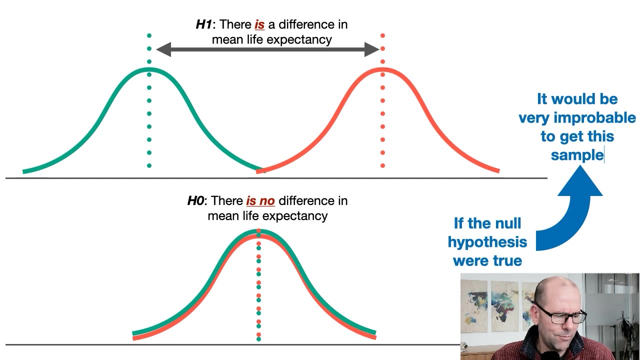 then how likely would it be that we would get a sample from the population that shows a difference that we're seeing or greater? What is the probability of that? If we find that that is very improbable- and we decide up front, by the way, we decide up front what we consider, what the threshold for what we would consider to be very improbable, what we mean by very- and we often use 5% if it's 5% or less in terms of likelihood or probability- if it would be very improbable to get a sample like we've gotten, if the null hypothesis were true. 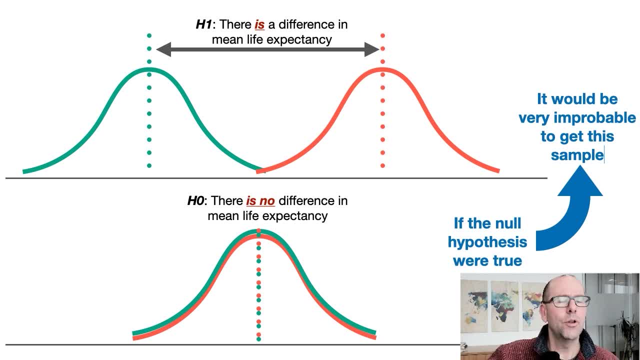 and it would be very improbable to get the sample, but we have gotten the sample. we can then make the inference that the null hypothesis must in fact be incorrect, That this assumption that there's no difference, that that's incorrect. We can reject that. 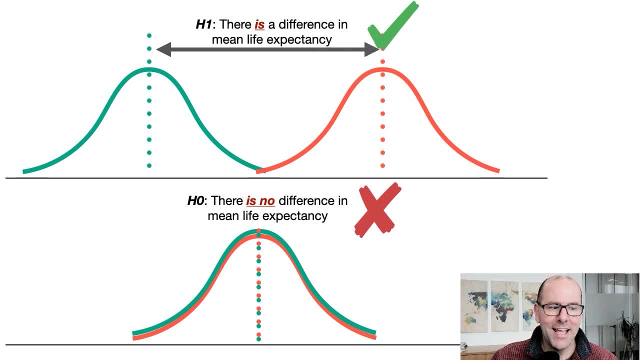 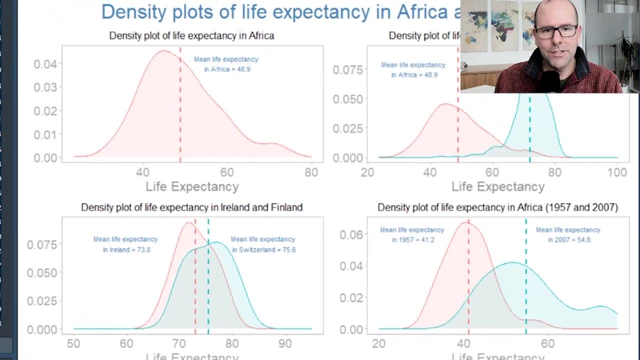 and we can accept the fact that there is in fact a difference and that our sample data is statistically significant, And that's how hypothesis testing works. So the first example here at the top on the left is a single sample t-test. In other words, we've just got one sample. in this case, we've just got life. 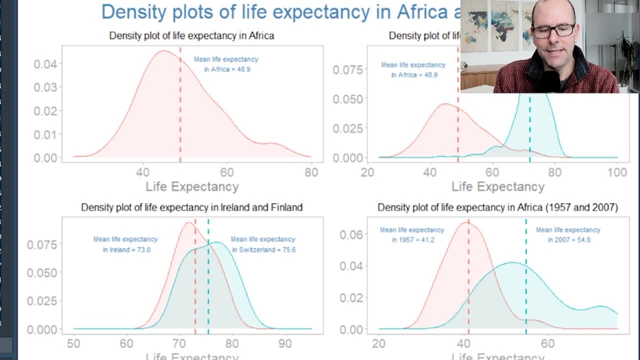 expectancy in Africa. so we've just taken Africa, we've got life expectancy. we don't have two populations, we've got one population, it's just Africa, and we've got a presumed life expectancy or presumed mean. It could be for any old reason, it could be any. 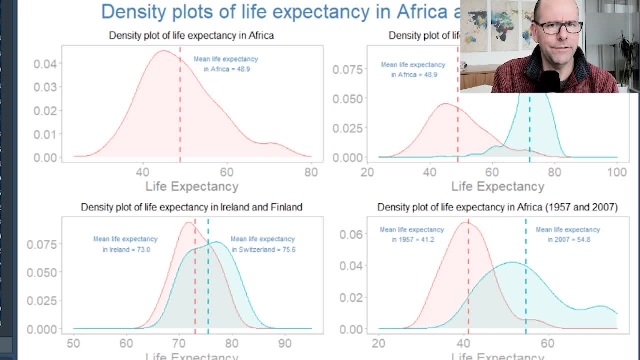 reason why we believe that the life expectancy should be 50 or should be 55, it could be any number- and we would ask the question: is the sample that we've got 48.9 years? is that statistically significantly different from that presumed mean or that presumed population mean? 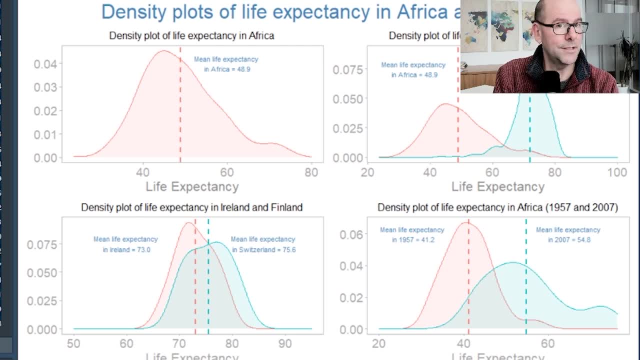 And then you get- you basically get a p-value. if that p-value is less than 0.05 or 5%- if that's the number that you've chosen as a threshold- it could be different. Then, if it's less than that threshold and it's. 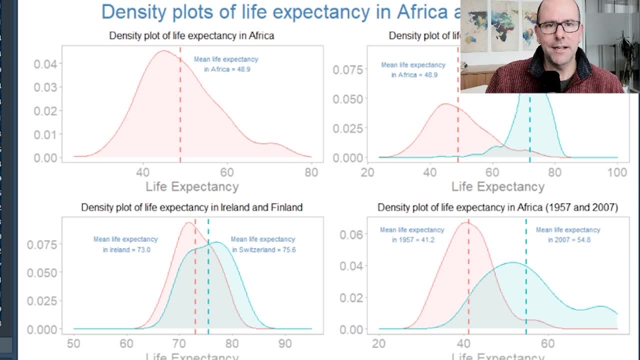 usually 0.05, then we can reject the null hypothesis that the average is whatever it is that we assumed it to be, and we can accept the fact that the sample mean that we've gotten is statistically significant. Okay, so that's the easiest example. If you understand that one. 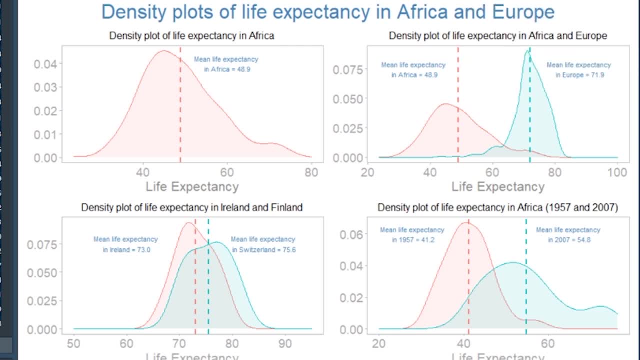 you'll understand the rest of these super duper easy. Let's keep going In these two examples- and I've got two here just to illustrate the fact that there's two possible ways of asking this next kind of question. We've got life expectancy in Africa and in Europe. 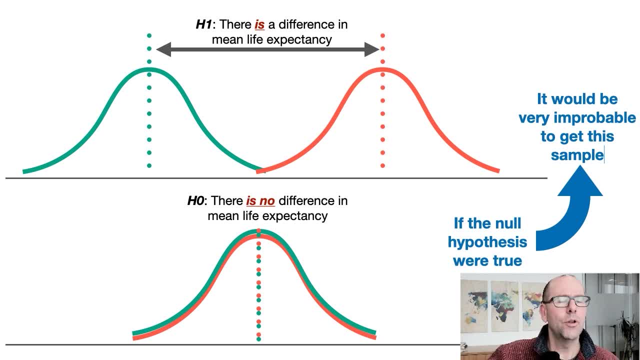 and it would be very improbable to get the sample, but we have gotten the sample. we can then make the inference that the null hypothesis must in fact be incorrect, That this assumption that there's no difference, that that's incorrect. We can reject that. 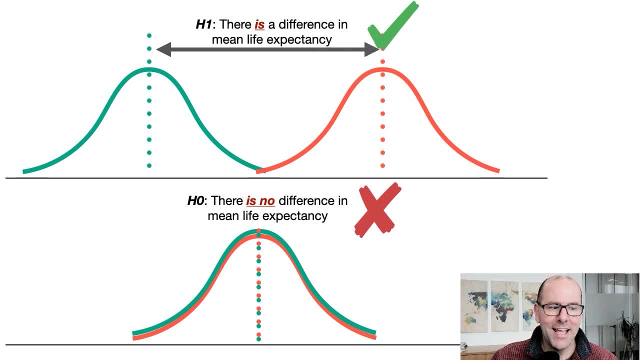 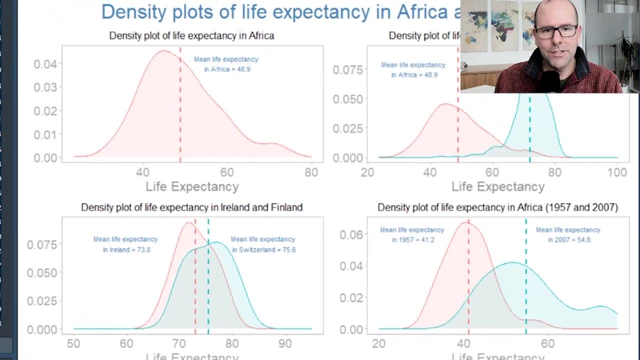 and we can accept the fact that there is in fact a difference and that our sample data is statistically significant, And that's how hypothesis testing works. So the first example here at the top on the left is a single sample t-test. In other words, we've just got one sample. in this case, we've just got life. 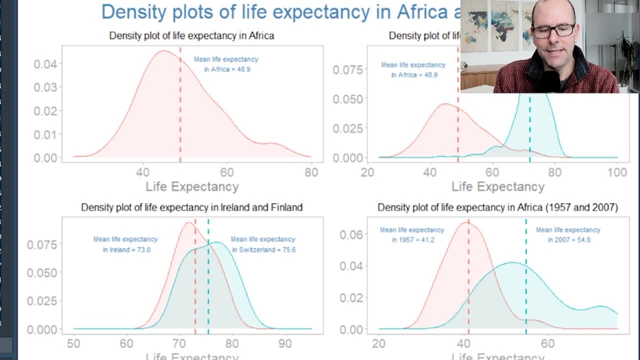 expectancy in Africa. so we've just taken Africa, we've got life expectancy. we don't have two populations, we've got one population, it's just Africa, and we've got a presumed life expectancy or presumed mean. It could be for any old reason, it could be any. 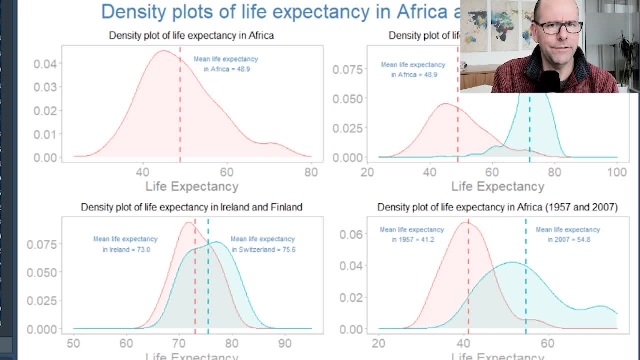 reason why we believe that the life expectancy should be 50 or should be 55, it could be any number- and we would ask the question: is the sample that we've got 48.9 years? is that statistically significantly different from that presumed mean or that presumed population mean? 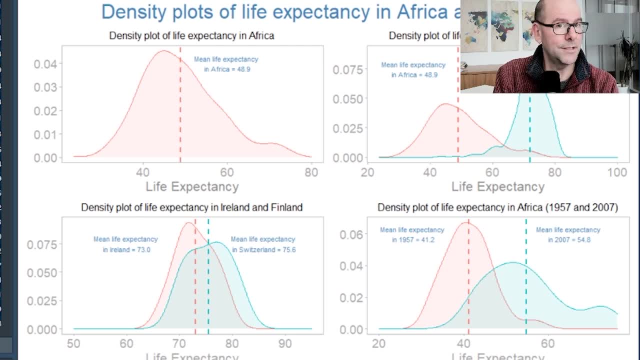 And then you get- you basically get a p-value. if that p-value is less than 0.05 or 5%- if that's the number that you've chosen as a threshold- it could be different. Then, if it's less than that threshold and it's. 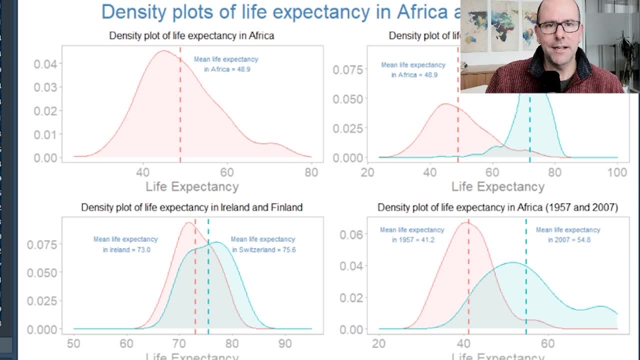 usually 0.05, then we can reject the null hypothesis that the average is whatever it is that we assumed it to be, and we can accept the fact that the sample mean that we've gotten is statistically significant. Okay, so that's the easiest example. If you understand that one. 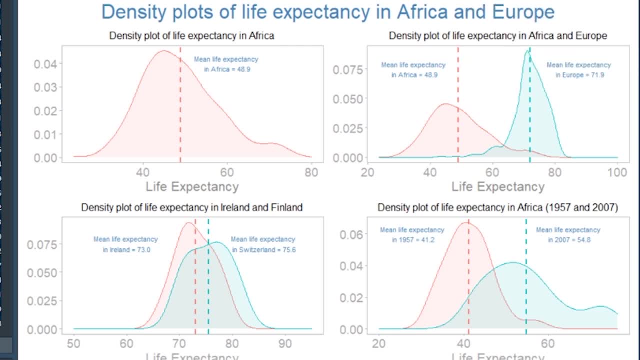 you'll understand the rest of these super duper easy. Let's keep going In these two examples- and I've got two here just to illustrate the fact that there's two possible ways of asking this next kind of question. We've got life expectancy in Africa and in Europe. 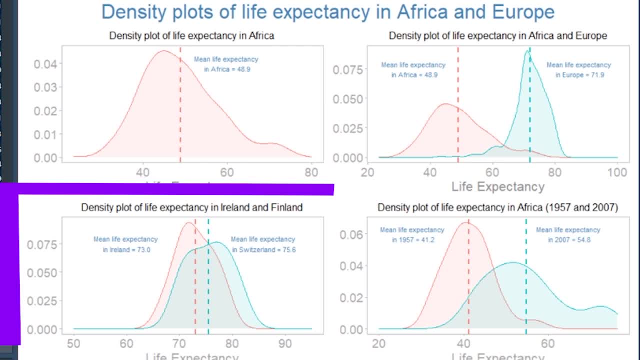 in the top right-hand corner, and we've got life expectancy in Ireland and in Switzerland at the bottom left over here. Now the reason I've got two here is just to highlight the fact that there's two ways of doing this. We could ask the question: is there a difference? without specifying in which? 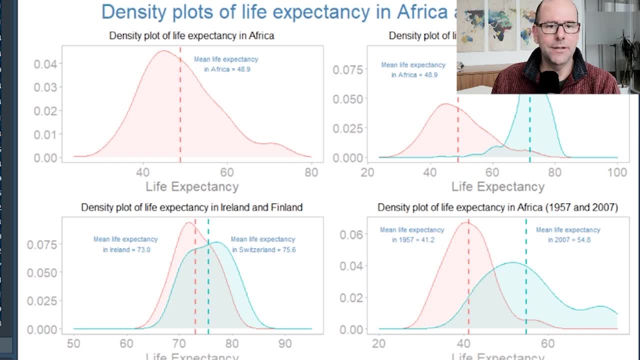 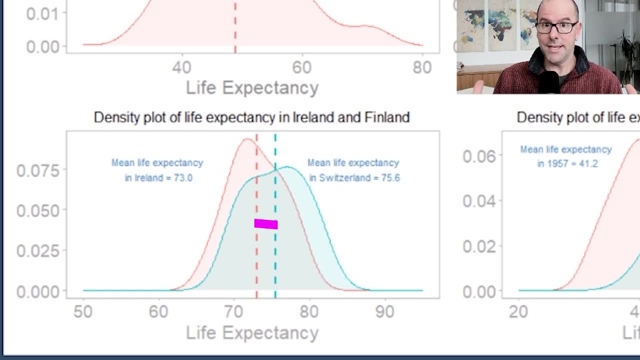 direction. So is there a difference, for example, between the life expectancy in Ireland and the life expectancy in Switzerland? And we might say: look, we don't know in which direction the difference might be. We're just asking: are they the same or are they different? Is the difference? 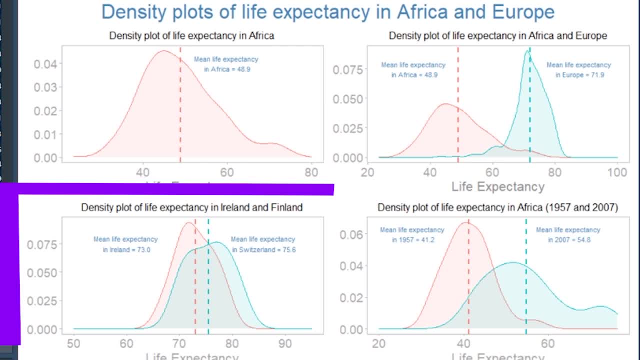 in the top right-hand corner, and we've got life expectancy in Ireland and in Switzerland at the bottom left over here. Now the reason I've got two here is just to highlight the fact that there's two ways of doing this. We could ask the question: is there a difference? without specifying in which? 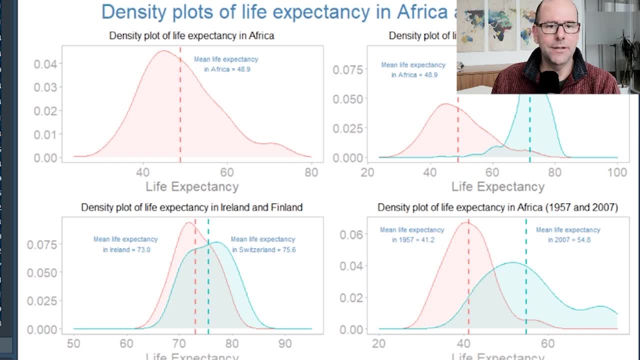 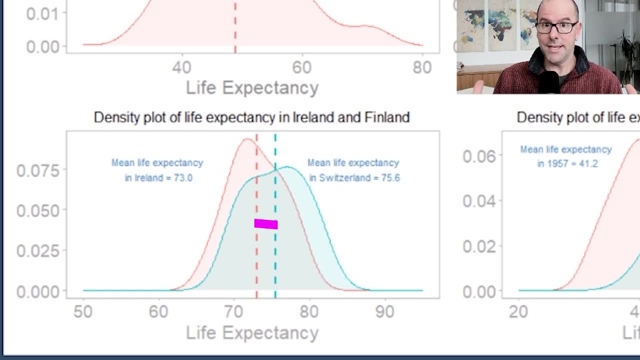 direction. So is there a difference, for example, between the life expectancy in Ireland and the life expectancy in Switzerland? And we might say: look, we don't know in which direction the difference might be. We're just asking: are they the same or are they different? Is the difference? 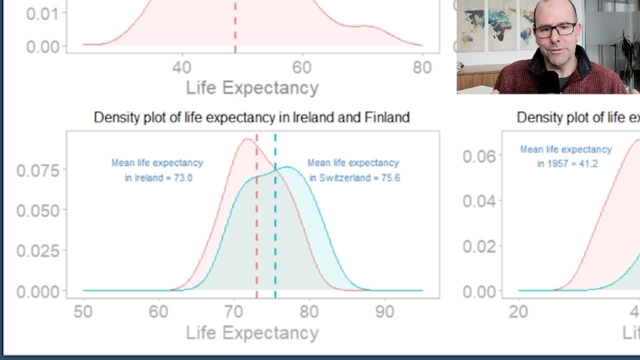 that we're seeing here statistically significant? Would we expect to see a difference of this magnitude or more if it were the case that, in the scenario of the null hypothesis that in fact Ireland and Switzerland have the exact same life expectancy, And if that probability is less than? 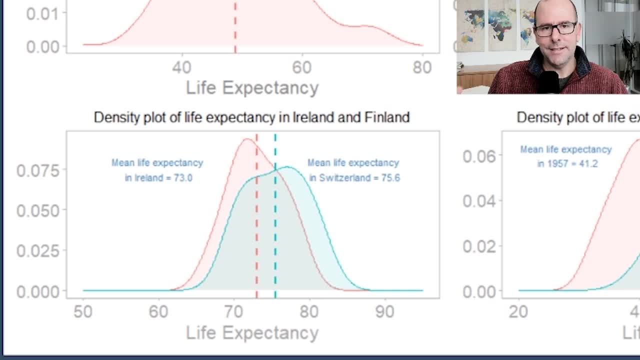 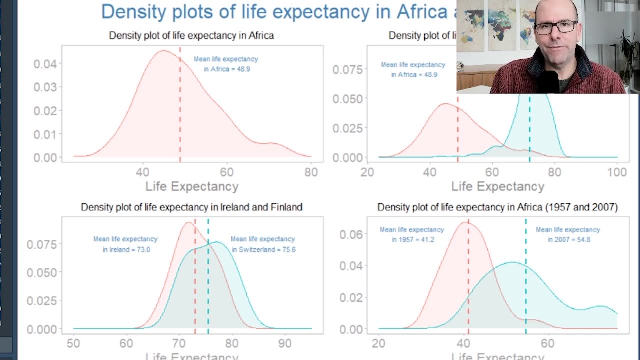 0.05,. if that's our threshold, then we would say that it is statistically significant. We reject the notion that they've got the same life expectancy and we accept the fact that a life expectancy, that this is statistically significant. We could approach the exact same problem in a slightly 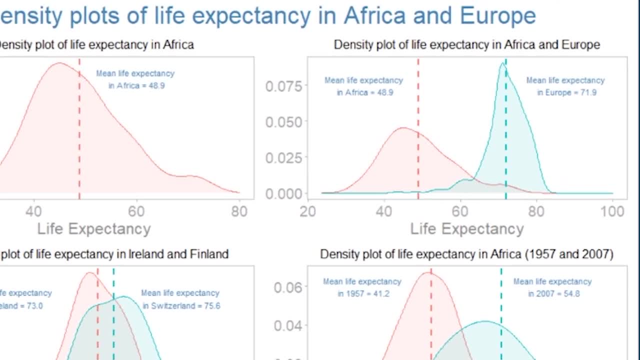 different way And let's use Africa and Europe for that. We could say: look, we want to ask the question: is it statistically significant that Africa has a life expectancy less than Europe of this magnitude? So we might go into the question: is there a difference between the two? 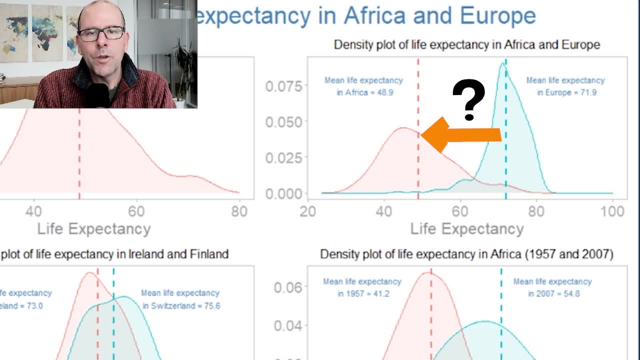 And we might say: look, we don't know in which direction the difference between the two. We know that Africa has got a life expectancy less than Europe. We're asking: is a difference of this magnitude statistically significant? So we're not asking: is there a difference in any? 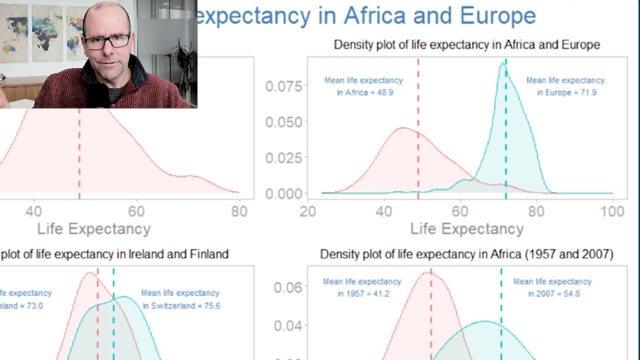 direction. We're saying: we think there is a difference. We're asking: is the life expectancy in Africa less than Europe by this magnitude or more, And is that statistically significant? And under those conditions, we're asking: is the life expectancy in Africa less than Europe by this? 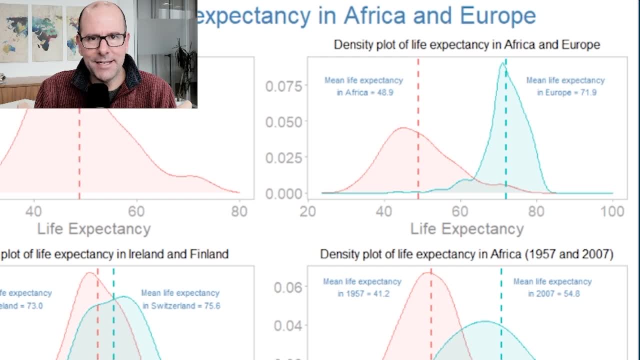 magnitude And under those circumstances you do a one-tailed t-test. Does that make sense? Two-tailed if you're saying is there a difference in any direction. One-tailed if you're saying is there a difference in a particular direction. Okay, you got it. And in both cases the null. 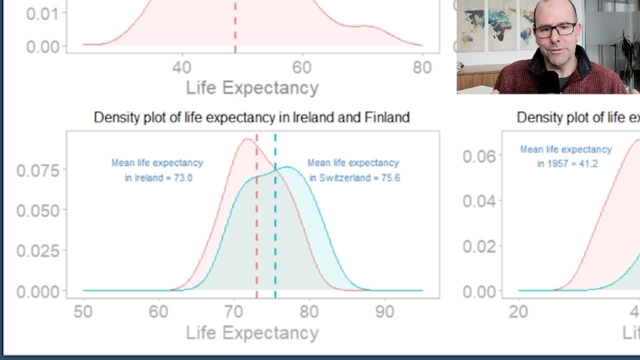 that we're seeing here statistically significant? Would we expect to see a difference of this magnitude or more if it were the case that, in the scenario of the null hypothesis that in fact Ireland and Switzerland have the exact same life expectancy, And if that probability is less than? 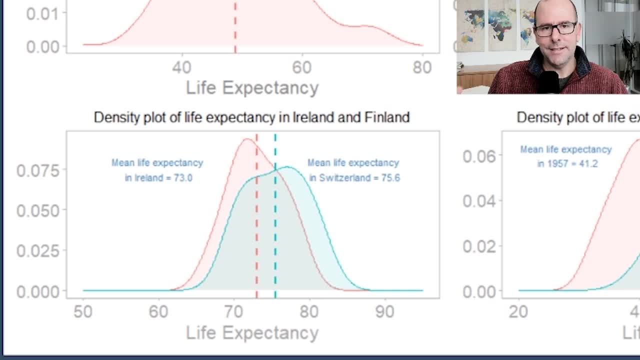 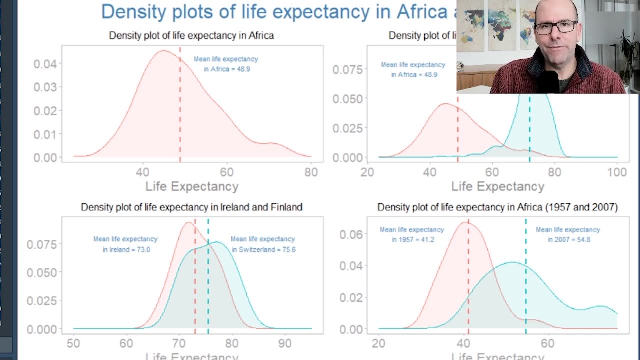 0.05,. if that's our threshold, then we would say that it is statistically significant. We reject the notion that they've got the same life expectancy and we accept the fact that a life expectancy, that this is statistically significant. We could approach the exact same problem in a slightly 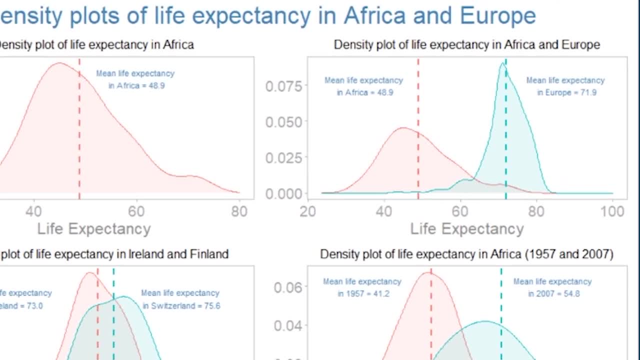 different way And let's use Africa and Europe for that. We could say: look, we want to ask the question: is it statistically significant that Africa has a life expectancy less than Europe of this magnitude? So we might go into the question: is there a difference between the two? 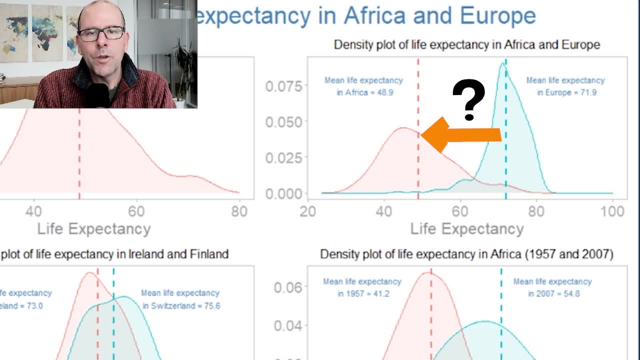 And we might say: look, we don't know in which direction the difference between the two. We know that Africa has got a life expectancy less than Europe. We're asking: is a difference of this magnitude statistically significant? So we're not asking: is there a difference in any? 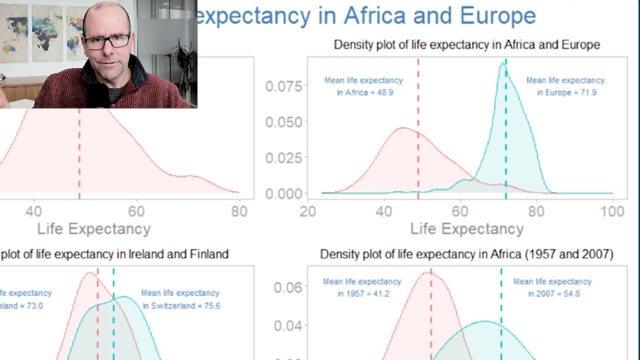 direction. We're saying: we think there is a difference. We're asking: is the life expectancy in Africa less than Europe by this magnitude or more, And is that statistically significant? And under those conditions, we're asking: is the life expectancy in Africa less than Europe by this? 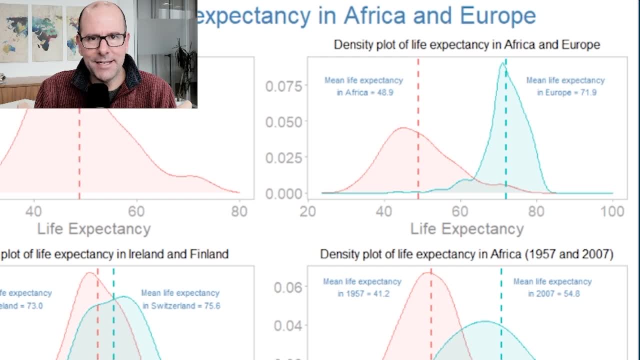 magnitude And under those circumstances you do a one-tailed t-test. Does that make sense? Two-tailed if you're saying is there a difference in any direction. One-tailed if you're saying is there a difference in a particular direction. Okay, you got it. And in both cases the null. 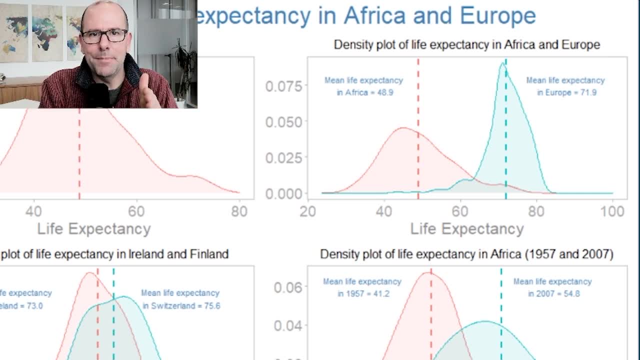 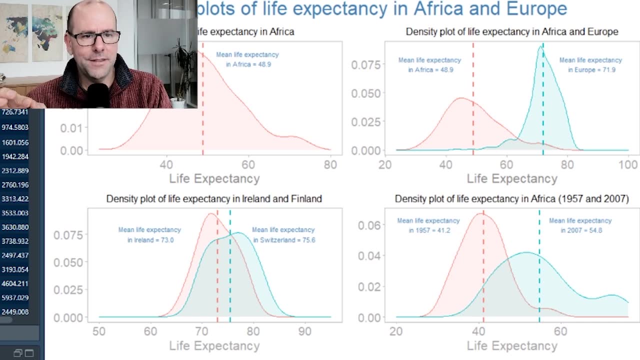 hypothesis is that both populations have got the same mean that there's no difference between the life expectancy in the two populations. Now here's the last example, And this is what I want you to understand. This is a paired t-test, So we've got a one-tailed and a two-tailed t-test. 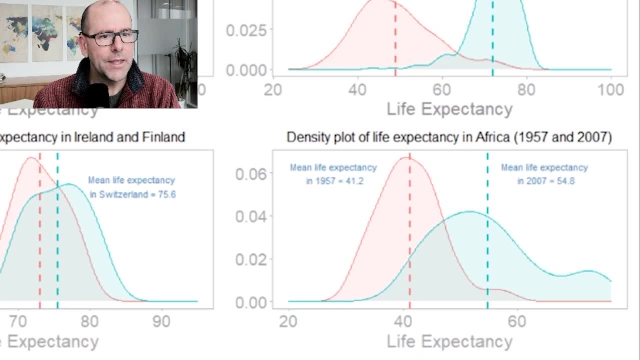 A paired t-test, and this illustrates it quite nicely. We've got a life expectancy in Africa in 1957, and then the life expectancy in Africa in 2007.. So for each sample, for each observation in the 1957, there is a counterpart in 2007,, right? So in Africa in 1957, one of the examples 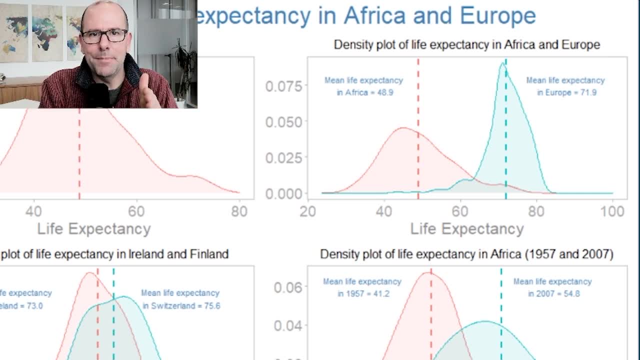 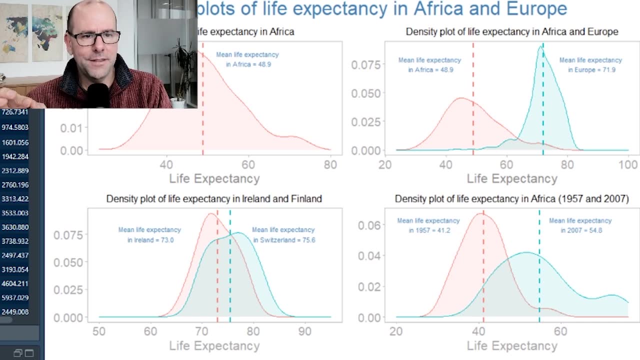 hypothesis is that both populations have got the same mean that there's no difference between the life expectancy in the two populations. Now here's the last example, And this is what I want you to understand. This is a paired t-test, So we've got a one-tailed and a two-tailed t-test. 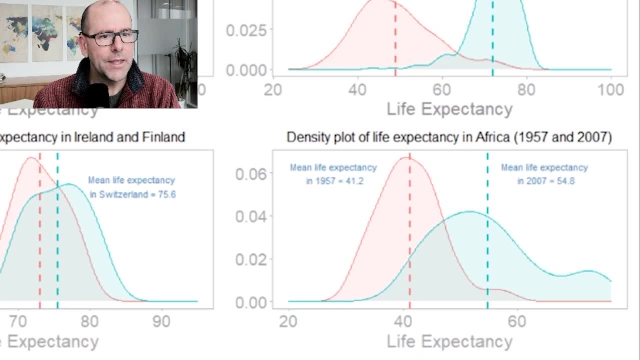 A paired t-test, and this illustrates it quite nicely. We've got a life expectancy in Africa in 1957, and then the life expectancy in Africa in 2007.. So for each sample, for each observation in the 1957, there is a counterpart in 2007,, right? So in Africa in 1957, one of the examples 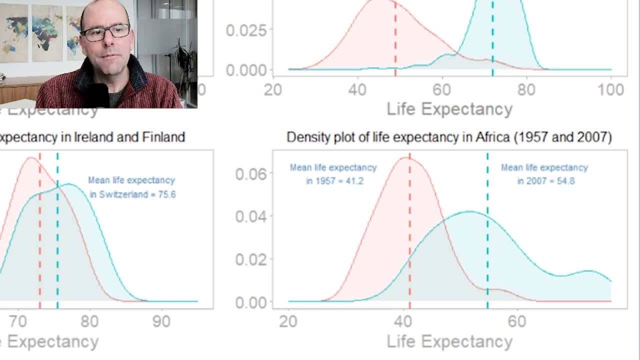 would be South Africa, There'd be a life expectancy. That's one of the observations. But in 2007, there would also be an observation that was South Africa, right, And there'd be a life expectancy there. Malawi in both cases. Zimbabwe in both samples. In other, 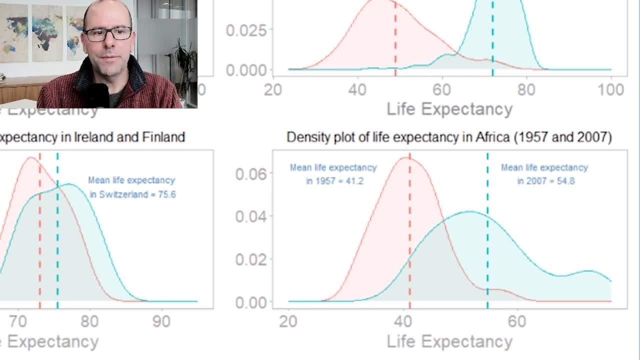 words, there are these pairs, There is a counterpart in each population And under those circumstances, you do a paired t-test And all of the principles, the exact same principles, apply, right? You can be one-sided, two-sided And, of course, the p-value of less than a 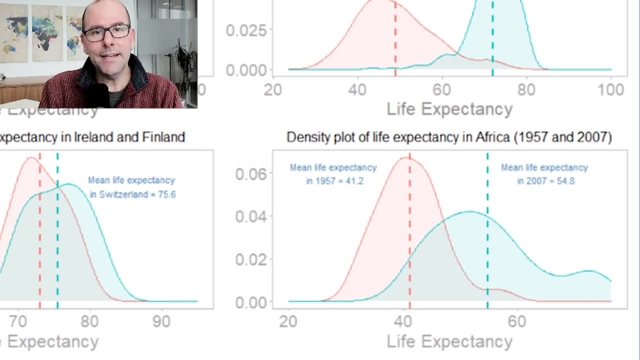 threshold that you determine up front. anything less than that threshold- if it's 5%- means that the null hypothesis gets rejected. The null hypothesis is that both of these have got the exact same life expectancy, the exact same mean, And if that's not the case, if we reject that. 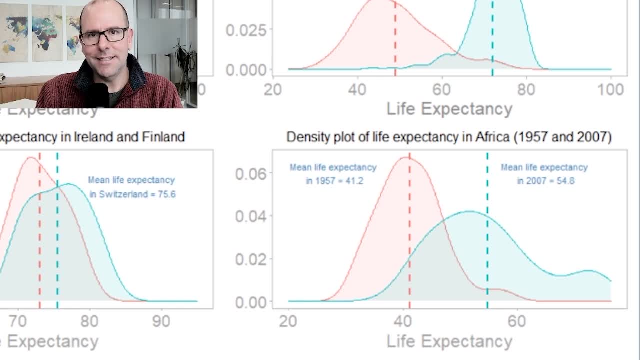 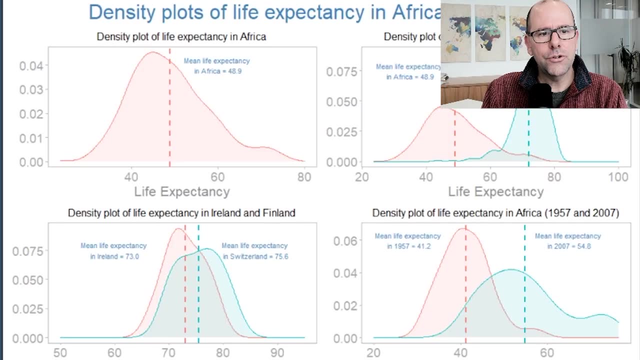 we can accept that the difference that we're seeing is statistically significant. All right, got it, Let's keep going. Next we're going to talk about ANOVA. So here we've got two means and a third. what do we do? We can't do three means. with a t-test, We would do an analysis of 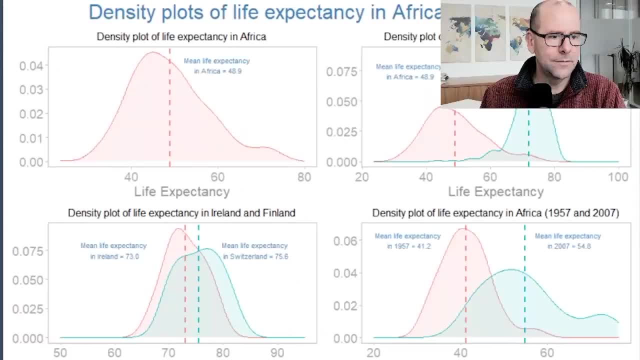 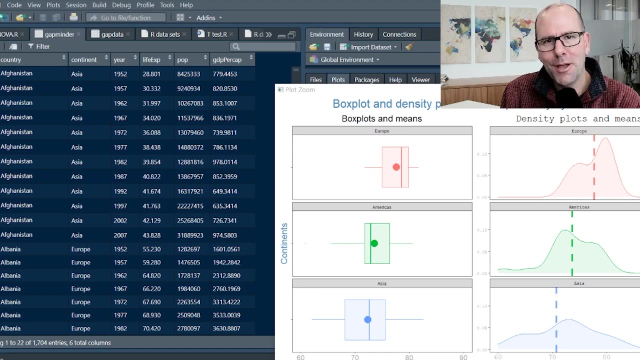 variance ANOVA. all right, So let's look at that next, Analysis of variance. we're trying to basically answer the same kind of question that we were with the t-test, but except now we've got three populations, three or more populations, and we wanted to compare the means right, The null. 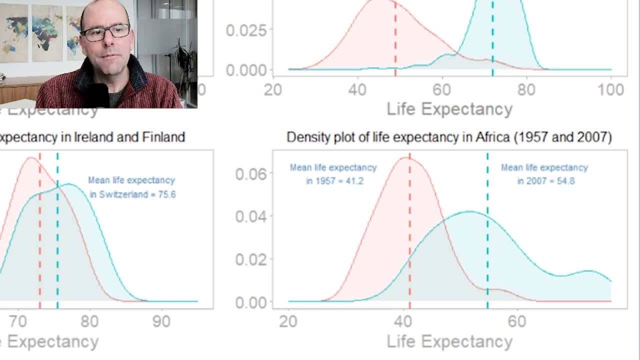 would be South Africa, There'd be a life expectancy. That's one of the observations. But in 2007, there would also be an observation that was South Africa, right, And there'd be a life expectancy there. Malawi in both cases. Zimbabwe in both samples. In other, 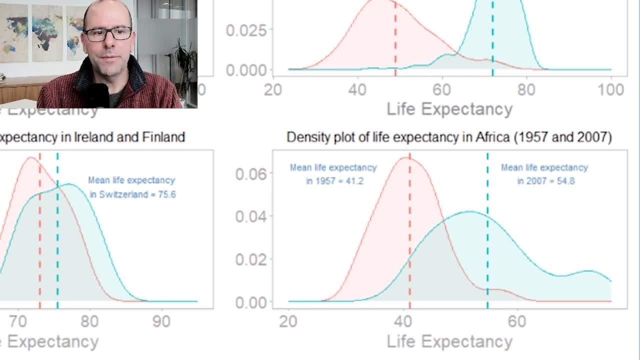 words, there are these pairs, There is a counterpart in each population And under those circumstances, you do a paired t-test And all of the principles, the exact same principles, apply, right? You can be one-sided, two-sided And, of course, the p-value of less than a 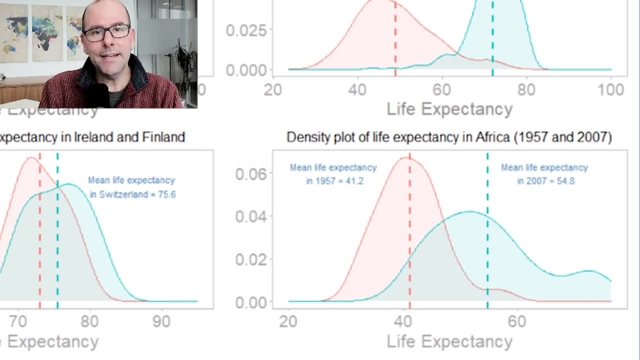 threshold that you determine up front. anything less than that threshold- if it's 5%- means that the null hypothesis gets rejected. The null hypothesis is that both of these have got the exact same life expectancy, the exact same mean, And if that's not the case, if we reject that. 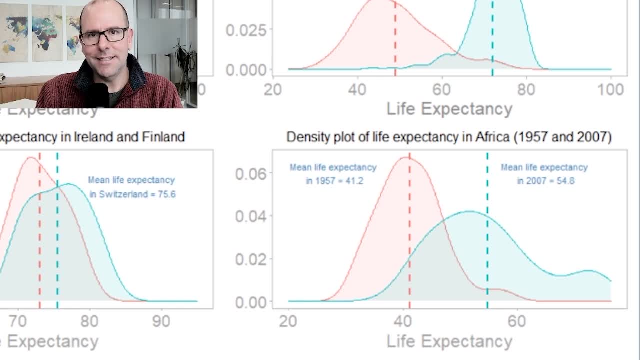 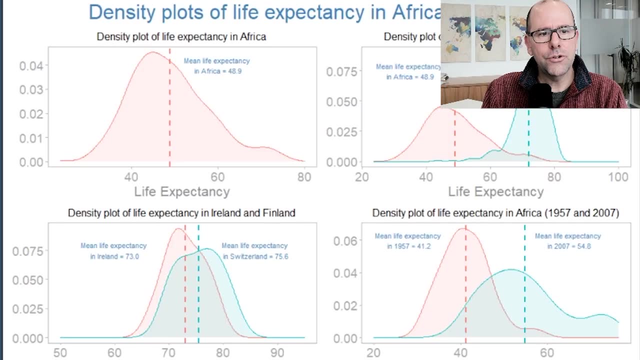 we can accept that the difference that we're seeing is statistically significant. All right, got it, Let's keep going. Next we're going to talk about ANOVA. So here we've got two means and a third. what do we do? We can't do three means. with a t-test, We would do an analysis of 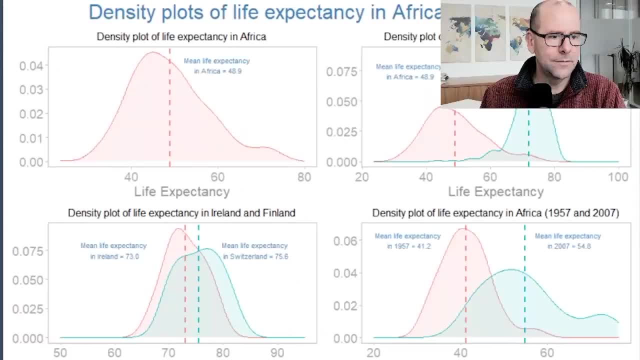 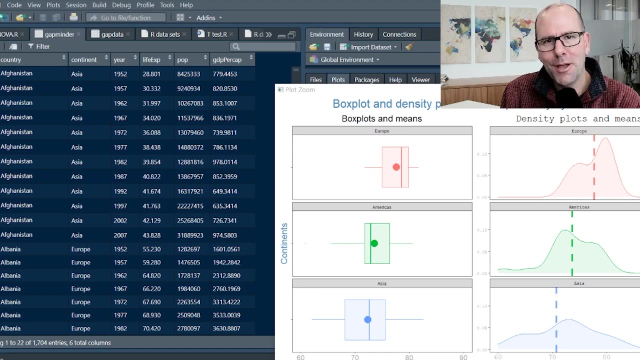 variance ANOVA. all right, So let's look at that next, Analysis of variance. we're trying to basically answer the same kind of question that we were with the t-test, but except now we've got three populations, three or more populations, and we wanted to compare the means right, The null. 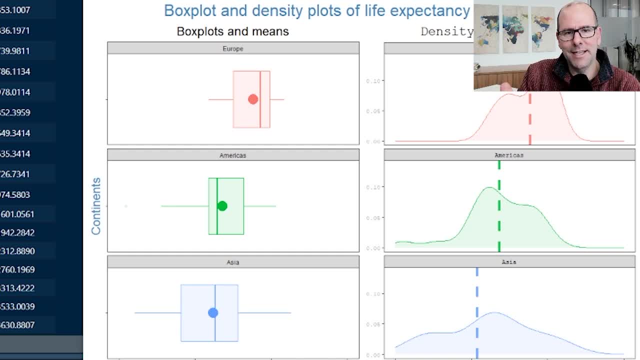 hypothesis is still the same, that the null hypothesis is that there are no differences in the means of these populations, And the alternative hypothesis is that in fact there is a difference, that the difference we're seeing is statistically significant. right, In this case I've used box plots and density plots. 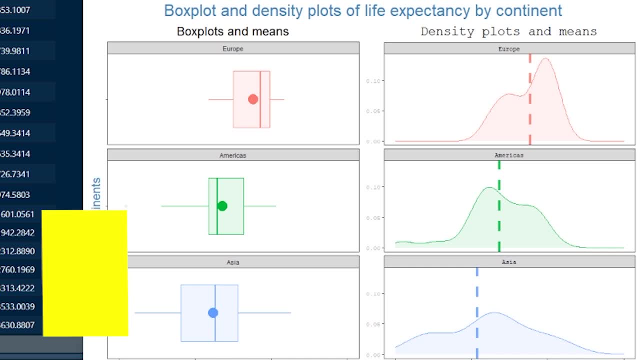 to illustrate the difference in means in three populations. We've got Europe, the Americas and Asia. This is taken from the Gapminder data. This is real data, so it's super-duper interesting And we're seeing here that the data is showing a difference in the means across these. 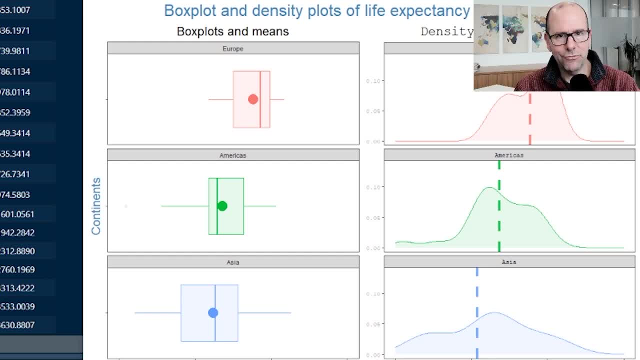 different population groups right. The question is: is that difference real? and if we do an ANOVA test it will show a p-value that's very small. But once you've done that right, you've done the ANOVA test, you've shown that there's a small p-value, we can reject the. 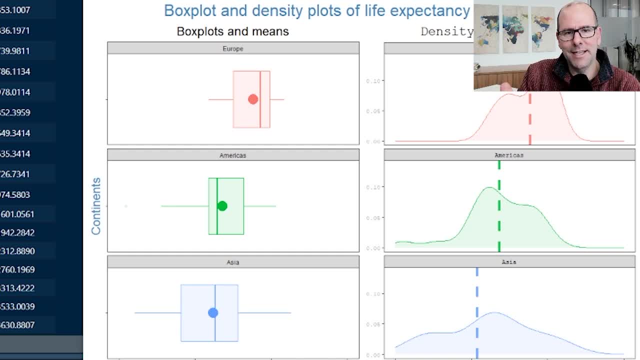 hypothesis is still the same, that the null hypothesis is that there are no differences in the means of these populations, And the alternative hypothesis is that in fact there is a difference, that the difference we're seeing is statistically significant. right, In this case I've used box plots and density plots. 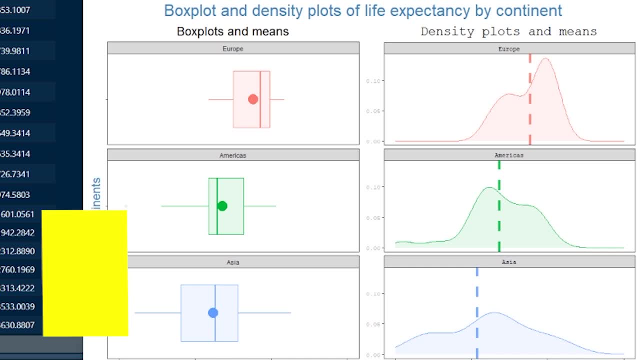 to illustrate the difference in means in three populations. We've got Europe, the Americas and Asia. This is taken from the Gapminder data. This is real data, so it's super-duper interesting And we're seeing here that the data is showing a difference in the means across these. 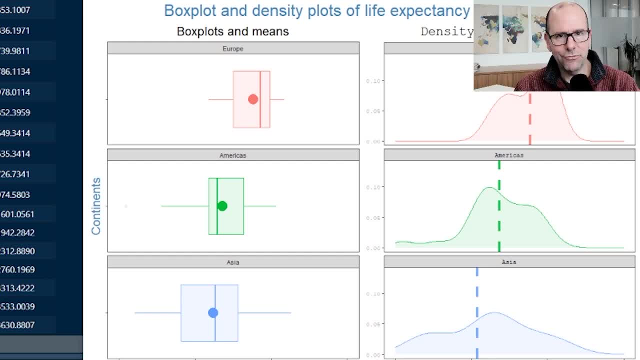 different population groups right. The question is: is that difference real? and if we do an ANOVA test it will show a p-value that's very small. But once you've done that right, you've done the ANOVA test, you've shown that there's a small p-value, we can reject the. 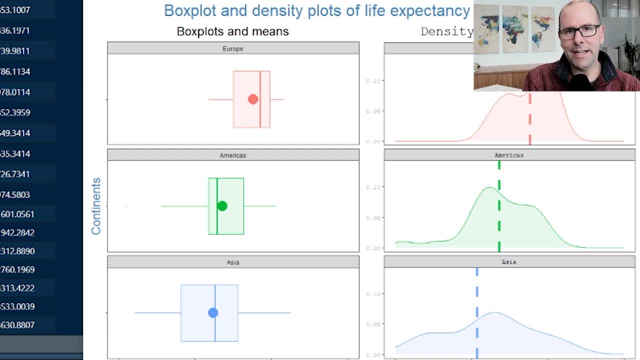 null hypothesis, which is that there's no difference in the means, we can accept the fact that there is some sort of statistical difference. How, then, do we tease out what's driving that difference? right, Because all that conclusion, all we can conclude from that, is that one of these populations 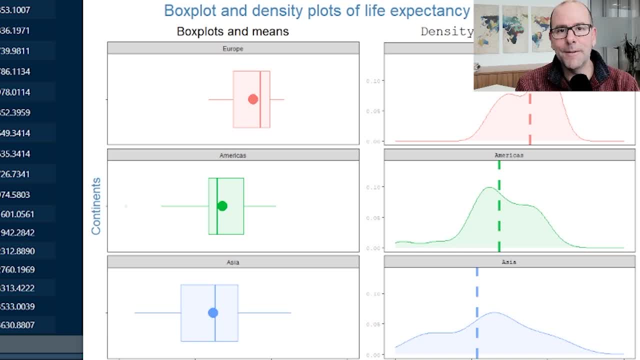 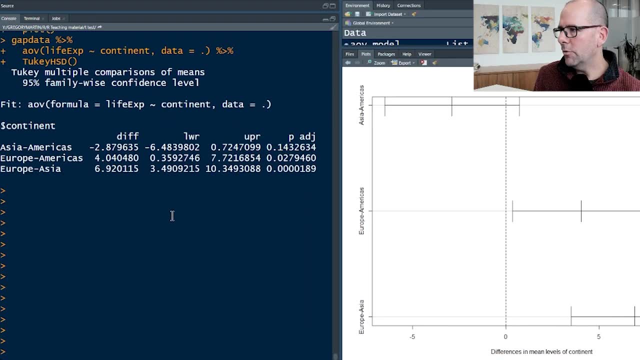 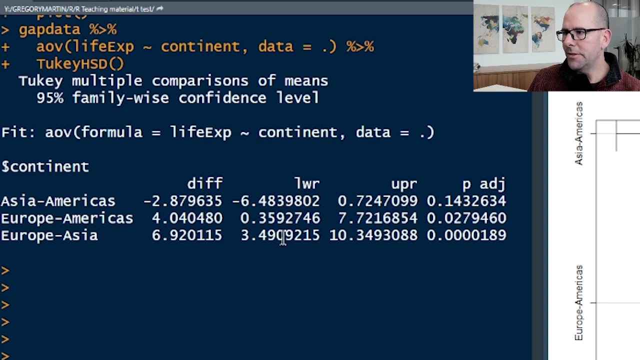 is different from the others, And sometimes there's. you know, you may have more than three here And you can do. there are ways of determining what's driving that difference, And what I've done here is I've fed our model into what's called a two-key multiple comparison of means, And it's taken each of the 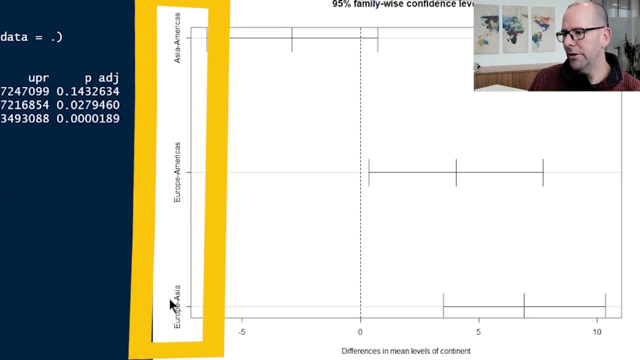 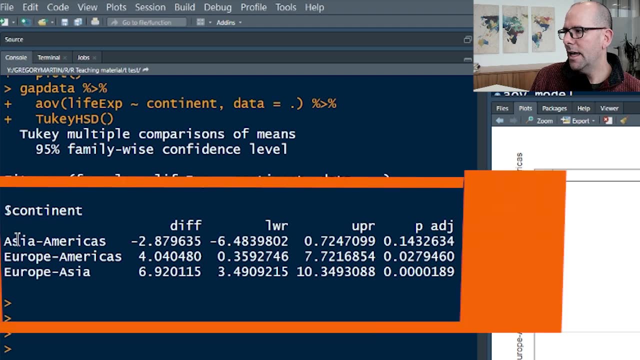 options. you know Asia and America, Europe and America and Europe and Asia and looked at them individually right, And if you look at the results of it, it's quite interesting because you can sort of see well between Asia and America. 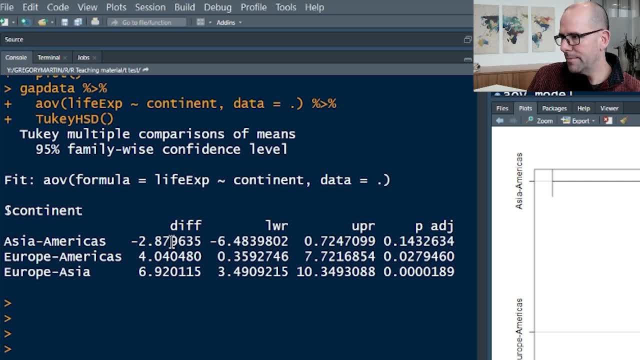 there's a difference of minus two or the difference of two, it doesn't really matter, the magnitude doesn't matter. But the confidence interval for that difference is between minus six and 0.72.. And here you can see it diagrammatically, that confidence interval. 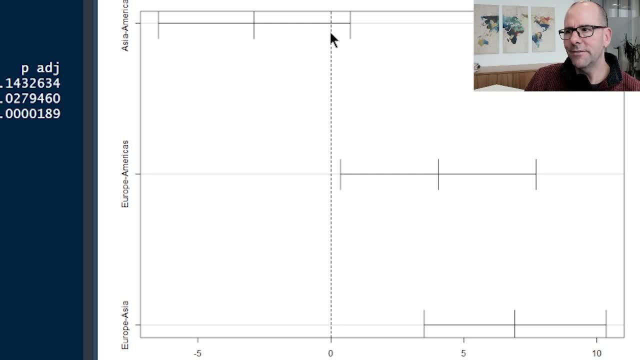 crosses the zero threshold, In other words, the confidence interval. the 95% confidence interval includes the possibility of a zero, which a zero means there's zero difference. In other words, it includes the possibility that there's no difference between those two population means. 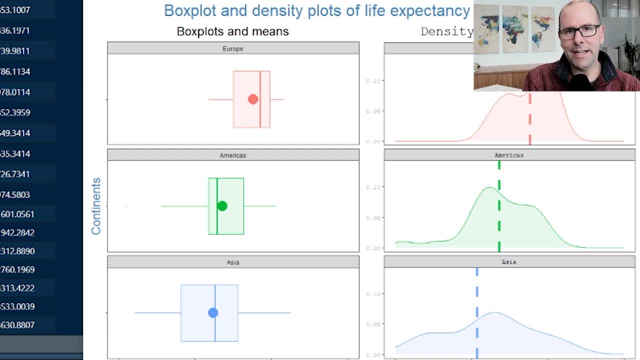 null hypothesis, which is that there's no difference in the means, we can accept the fact that there is some sort of statistical difference. How, then, do we tease out what's driving that difference? right, Because all that conclusion, all we can conclude from that, is that one of these populations 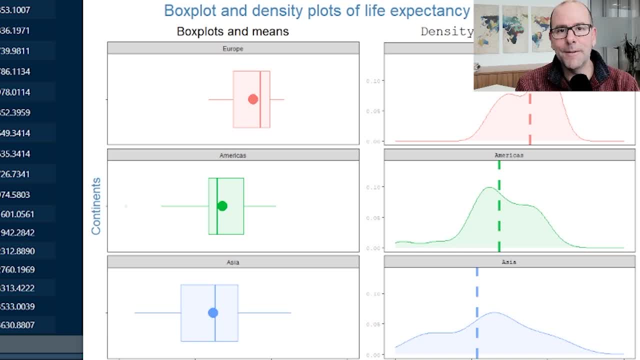 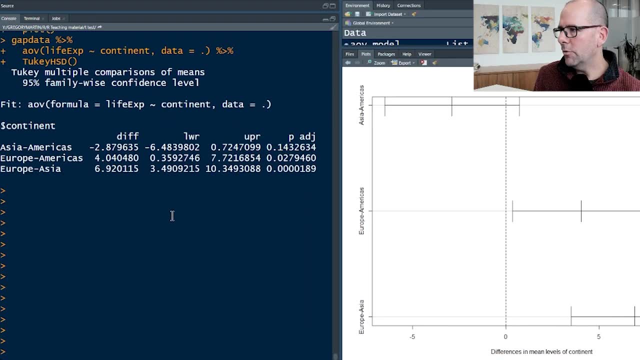 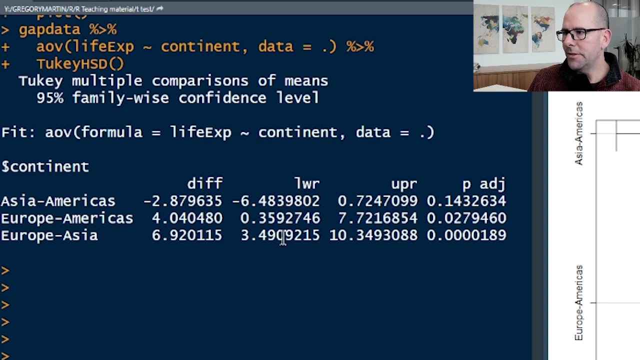 is different from the others, And sometimes there's. you know, you may have more than three here And you can do. there are ways of determining what's driving that difference, And what I've done here is I've fed our model into what's called a two-key multiple comparison of means, And it's taken each of the 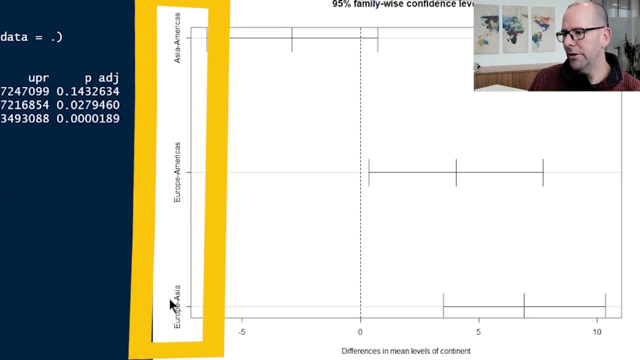 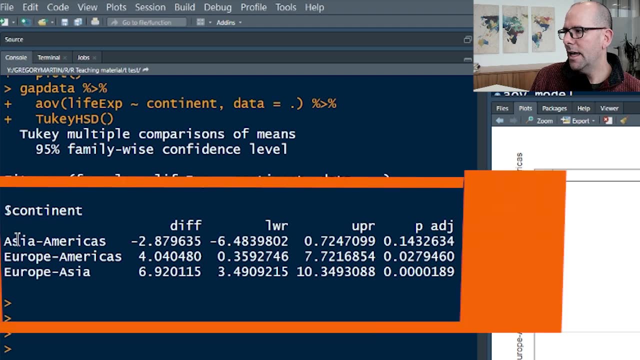 options. you know Asia and America, Europe and America and Europe and Asia and looked at them individually right, And if you look at the results of it, it's quite interesting because you can sort of see well between Asia and America. 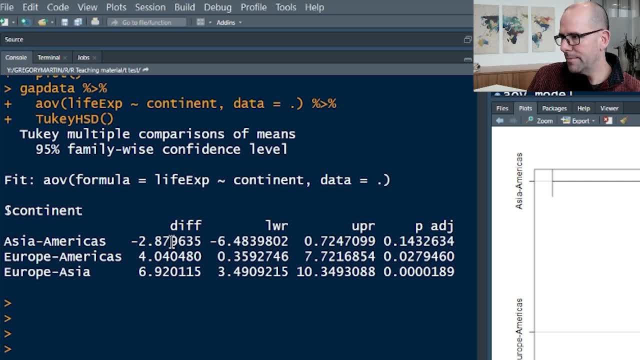 there's a difference of minus two or the difference of two, it doesn't really matter, the magnitude doesn't matter. But the confidence interval for that difference is between minus six and 0.72.. And here you can see it diagrammatically, that confidence interval. 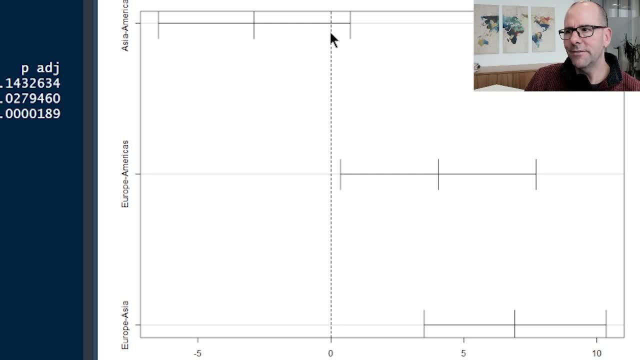 crosses the zero threshold, In other words, the confidence interval. the 95% confidence interval includes the possibility of a zero, which a zero means there's zero difference. In other words, it includes the possibility that there's no difference between those two population means. 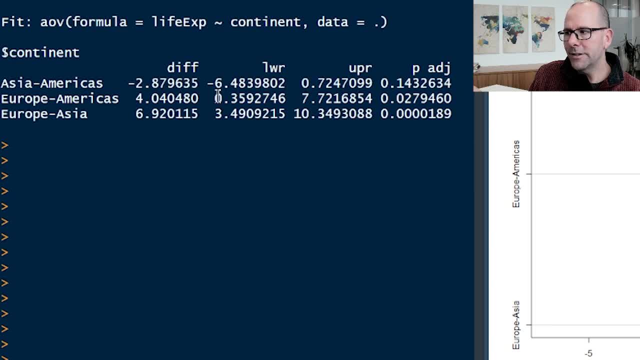 Europe and America. right, we've got a difference of four. the confidence interval does not include zero. it's from 0.3 to 7.2. And in Europe to Asia, again same story, quite a big difference. 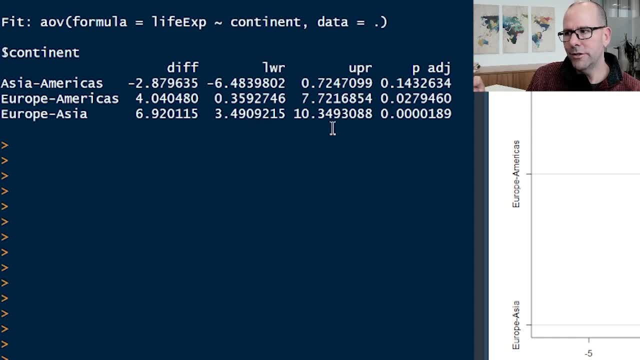 And the difference does not include the possibility of zero, of no difference And, as you would expect, the p-values, the adjusted p-values, bears that out. So in the Asia to America, where the confidence interval included zero, the p-value does not cross the threshold of 5% or less. 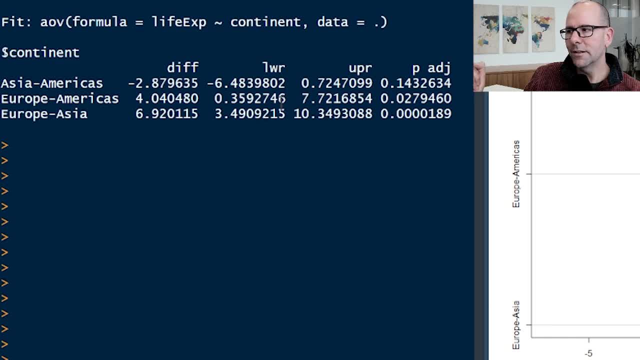 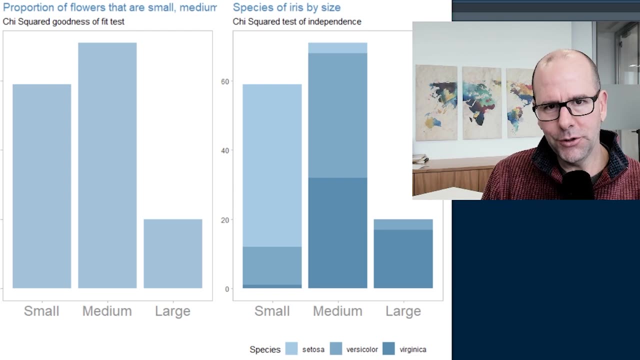 It's 0.14.. But the other two, where the confidence interval does not include zero, does not include the possibility of no difference. they both have small p-values, less than 0.05.. Okay, got it. Now let's talk about the chi-squared test. There's two of them, right? There's the goodness of fit. 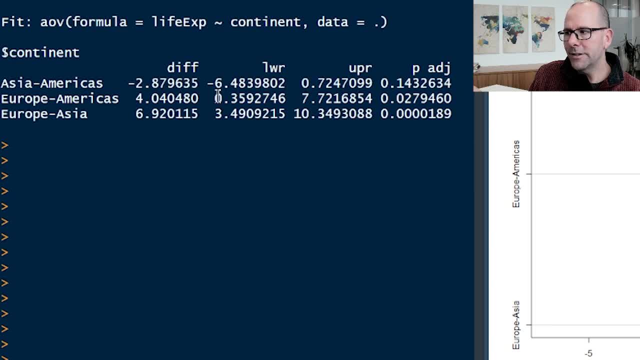 Europe and America. right, we've got a difference of four. the confidence interval does not include zero. it's from 0.3 to 7.2. And in Europe to Asia, again same story, quite a big difference. 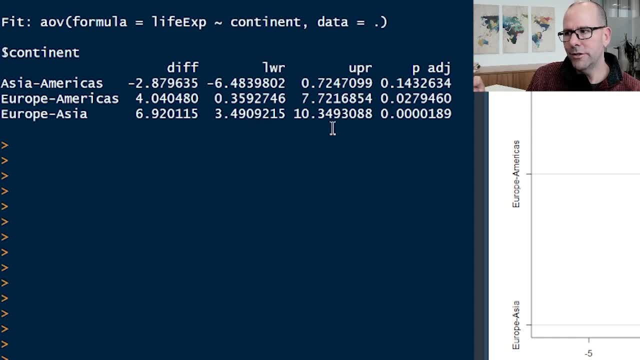 And the difference does not include the possibility of zero, of no difference And, as you would expect, the p-values, the adjusted p-values, bears that out. So in the Asia to America, where the confidence interval included zero, the p-value does not cross the threshold of 5% or less. 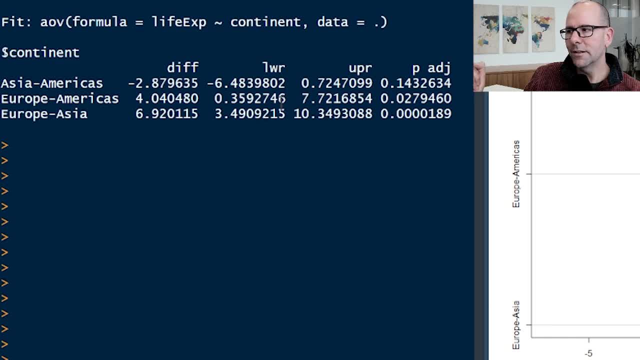 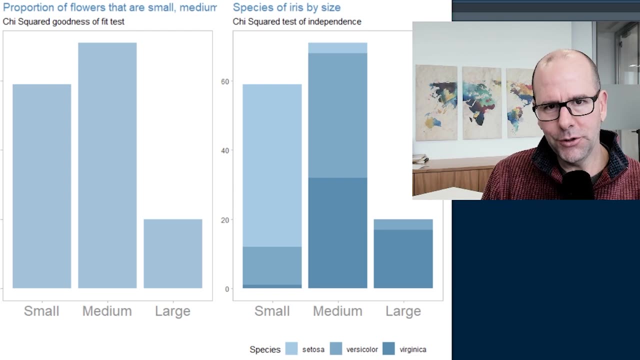 It's 0.14.. But the other two, where the confidence interval does not include zero, does not include the possibility of no difference. they both have small p-values, less than 0.05.. Okay, got it. Now let's talk about the chi-squared test. There's two of them, right? There's the goodness of fit. 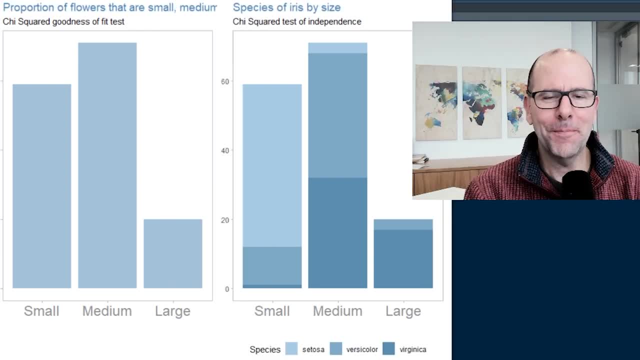 test and there's the chi-squared test of independence. Now, really, what we're looking at here is categorical variables and proportions of categorical variables, And this is a great test to kind of test the notion right. we're testing whether or not there in fact is a difference in 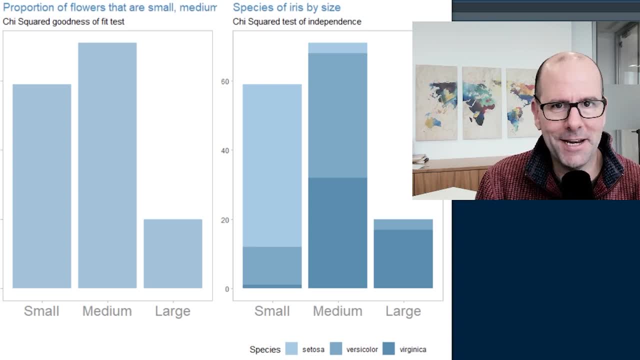 the proportions across the different categories. Okay, so let's have a look at that Right. so here we've got some flowers- these happen to be irises and we know that they come in. we've categorized them as small, medium and large And in the first instance, we could ask the question: are the 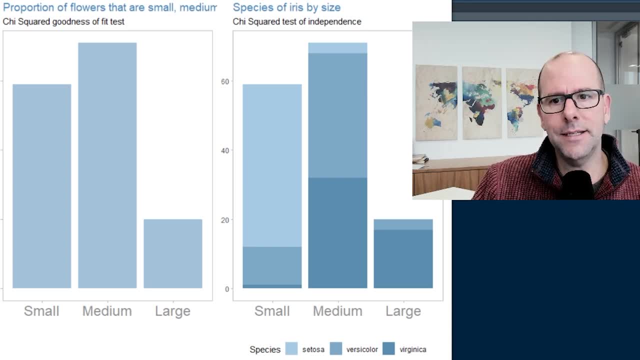 proportion of flowers that are small, medium, large the same. Do we expect to see the same number of small, medium and large flowers in a random sample that we take from a population And we answer that in the first instance we have a small, medium and large and large and a random. 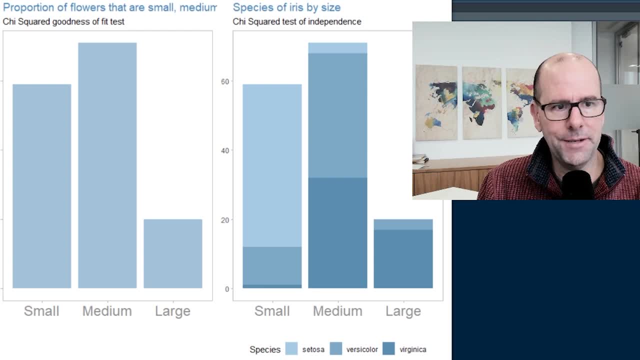 that question by doing a chi-squared goodness of fit test. let's have a look at that. and again, we're talking about hypothesis testing. in other words, if, if it were the case that there wasn't a difference in proportions, that would be our null hypothesis, right. our null hypothesis is that 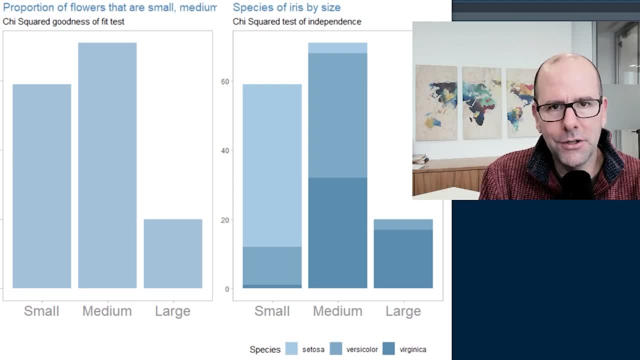 there's no difference in proportion, in the proportion of small, medium and large uh flowers. right, if that were true and we took a random sample and that random sample happened to show a difference in proportions as large as or bigger than the difference we're seeing now, we would consider if, if that, if, if that eventuality was considered to be extremely unlikely. 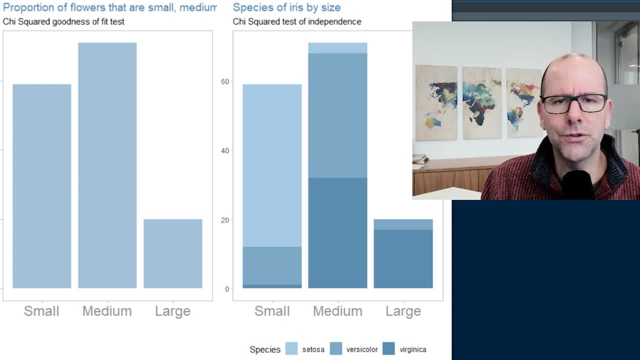 then we could reject the idea that they're all the same proportions and we could accept the fact that what we're seeing in the data is, in fact, statistically significant. what do we mean by extremely unlikely? well, we've got a cutoff point called the alpha value. that's the probability. 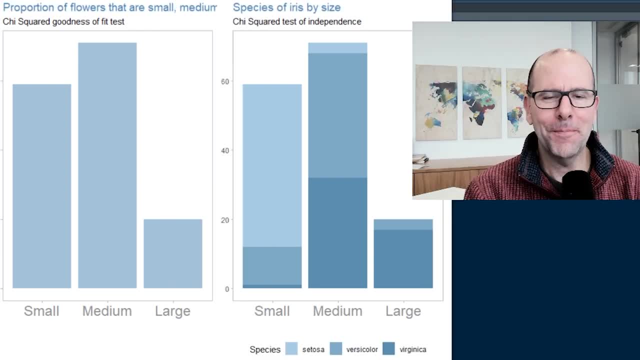 test and there's the chi-squared test of independence. Now, really, what we're looking at here is categorical variables and proportions of categorical variables, And this is a great test to kind of test the notion right. We're testing whether or not there in fact is a difference in 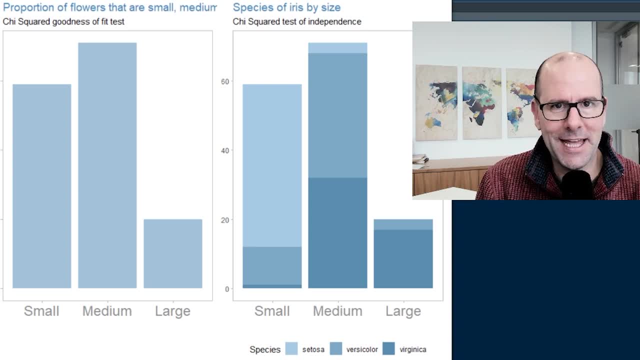 the proportions across the different categories. Okay, so let's have a look at that Right? so here we've got some flowers- These happen to be irises, and we know that they come in. we've categorized them as small, medium and large And in the first instance we could ask the question. 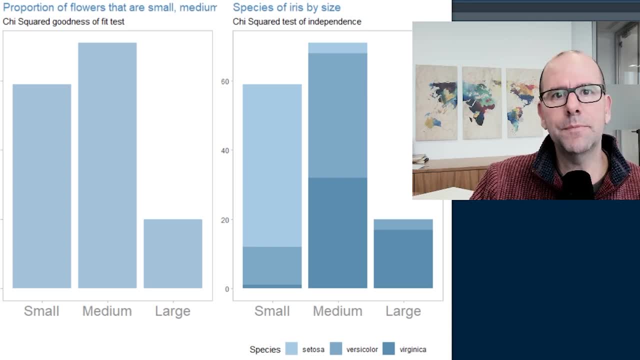 are the proportion of flowers that are small, medium and large the same? Do we expect to see the same number of small, medium and large flowers in a random sample that we take from the population And we answer the question: do we expect to see the same number of small, medium? 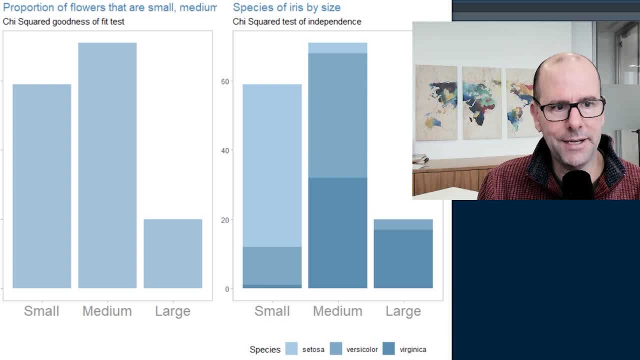 and large flowers in a random sample that we take from the population And we answer that question by doing a chi-squared goodness of fit test. Let's have a look at that. And again we're talking about hypothesis testing. In other words, if it were the case that there wasn't a difference in 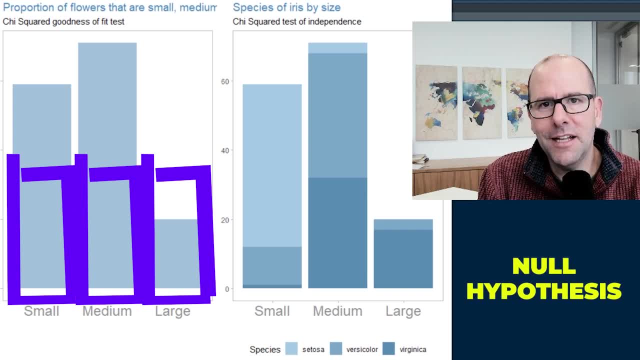 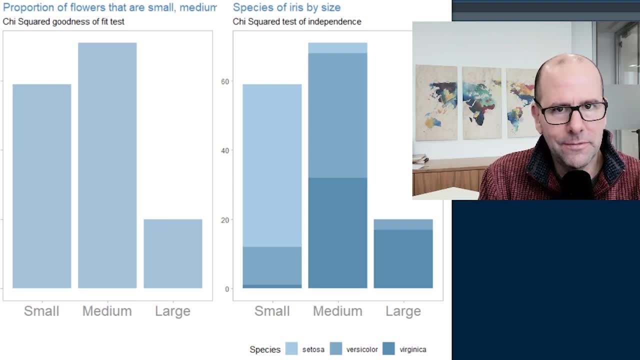 proportions. that would be our null hypothesis, right? Our null hypothesis is that there's no difference in proportion in the proportion of small, medium and large flowers. right, If that were true and we took a random sample and that random sample happened to show a difference in. 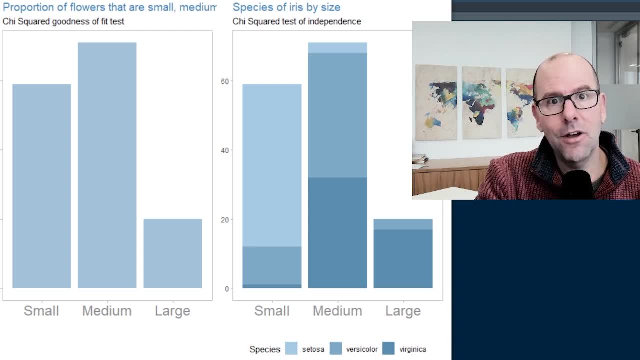 proportions as large as the proportion of small, medium and large flowers right, And we took a random sample and that random sample happened to show a difference in proportions as large as or bigger than the difference we're seeing now. we would consider if that eventuality was considered. 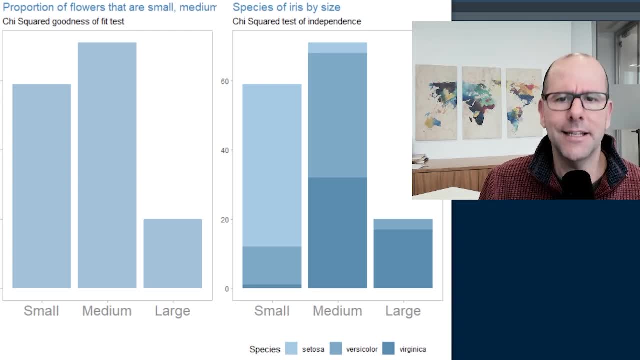 to be extremely unlikely. then we could reject the idea that they're all the same proportions and we could accept the fact that what we're seeing in the data is, in fact, statistically significant. What do we mean by extremely unlikely? Well, we've got a cutoff point called 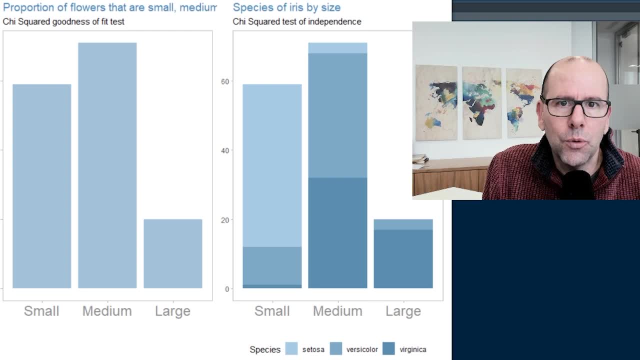 the alpha value. That's the probability. How small must that probability be for us to consider it to be Like unacceptably small, to the point that we wouldn't really believe that We wouldn't accept the null hypothesis to be true right? And usually we use 0.5, as we've talked about so many times in. 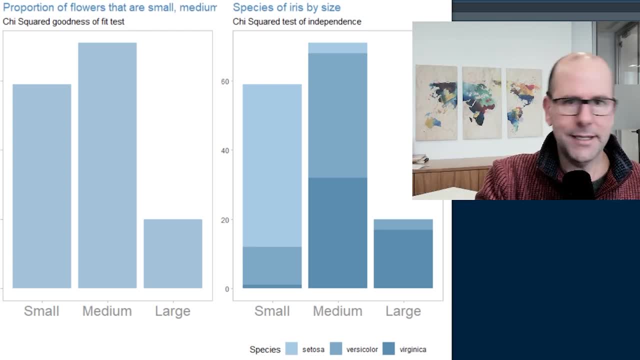 these videos. So we do a chi-square test. We take this data, we make a table, put it into the chi-square test and we get a p-value. That p-value is that probability If that p-value is less than the. 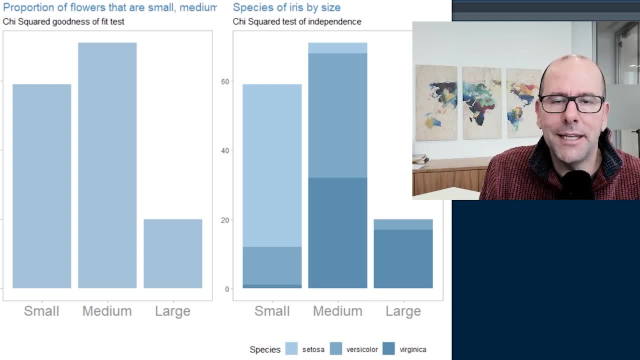 you know how small does. how small must that probability be for us to consider it to be not like like an unacceptably small, to the point that we wouldn't really believe that we wouldn't accept the null hypothesis to be true, right, and, and usually we use 0.5, as we've talked about. so 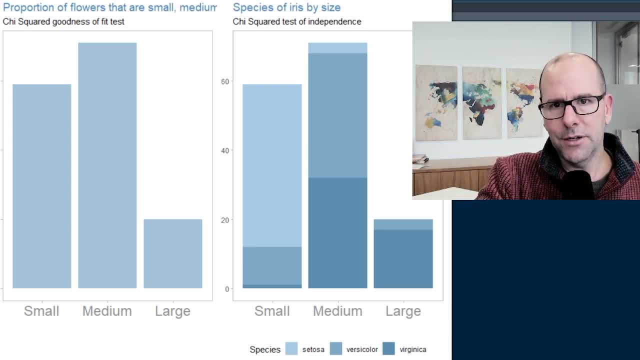 many times in these videos. so we do a chi-square test. we take the starter, we make a table, put it into the chi-square test and we get a p value. that p value is that probability if that p value is less than the threshold we talked about, usually 0.05, but it could be anything, depending on what it is. 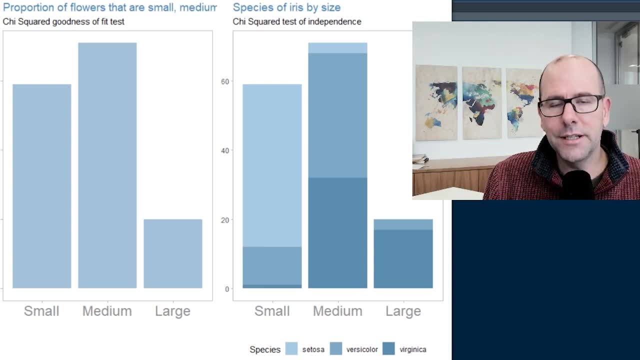 that you're trying to measure and how important your sort of discrimination is. if that p value is less than the threshold and we reject the null, we accept the alternative and we say that this difference that we're seeing in the data is in fact statistically significant and the exact same. 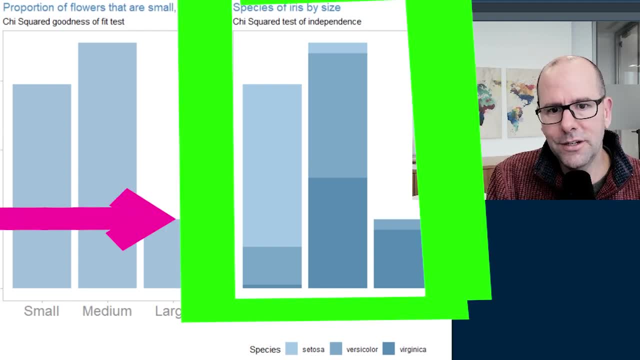 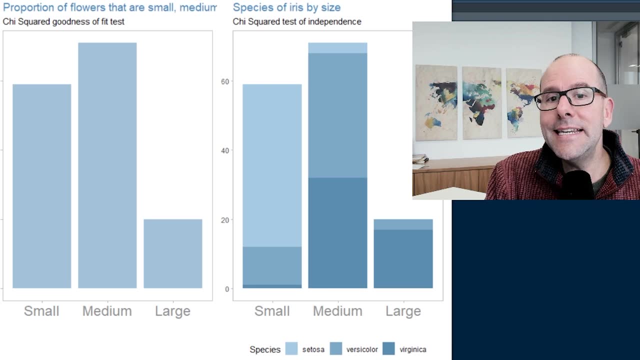 principle applies to the chi-square test of independence. we're asking the question: are the proportions of our species, are they in any way dependent or are they independent of the size of the flowers? is knowing the value you're knowing this is? does knowing the size of the flower tell us anything about the probability of a particular flower? 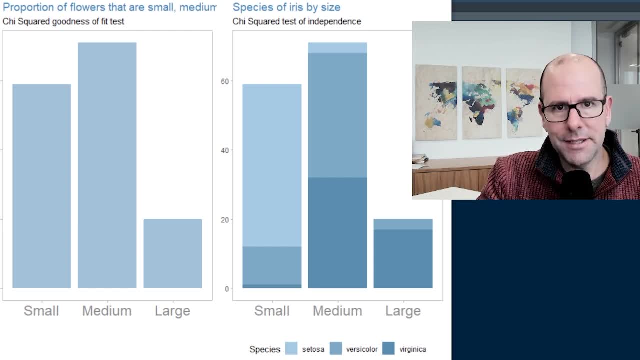 being in one of these species right, looking at these graphs, it seems that that is the case, but we need to demonstrate that statistically. so we do a chi, a chi-square test of independence and we get a p value. if the p value is very, very small beyond a predetermined threshold, remember it. 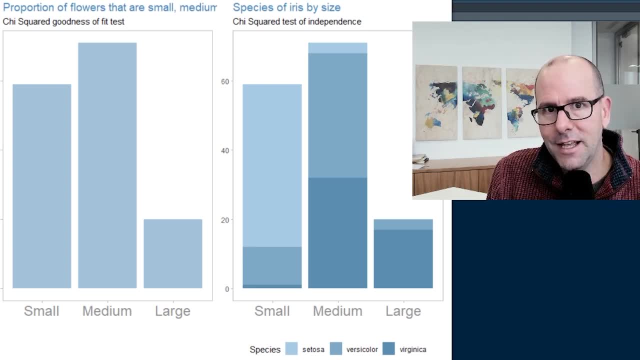 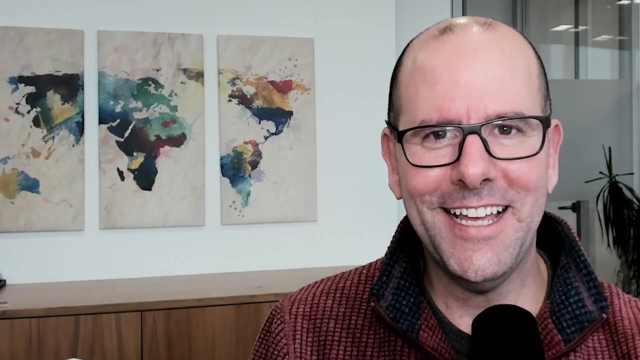 has to be predetermined. you can't do it retrospectively. that's p hacking, bad science. if it's, if the p value is very small, in other words, the probability ofames students, just questions, and questions on it, we see, is in fact statistically significant, right, that's the chi-squared test of independence. now stay, and 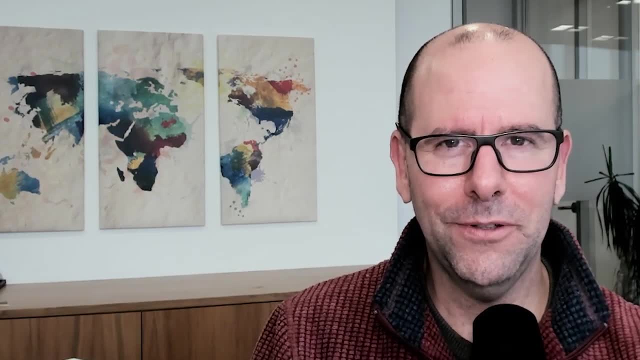 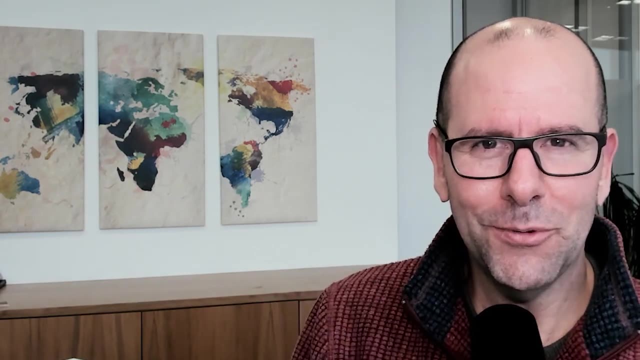 watch another video. share this video with people that you think might find it useful. subscribe to this channel if you haven't hit the bell notification if you want notification of future videos. take care, don't do drugs. always do your best, don't ever change. speak to you again soon. all the best. 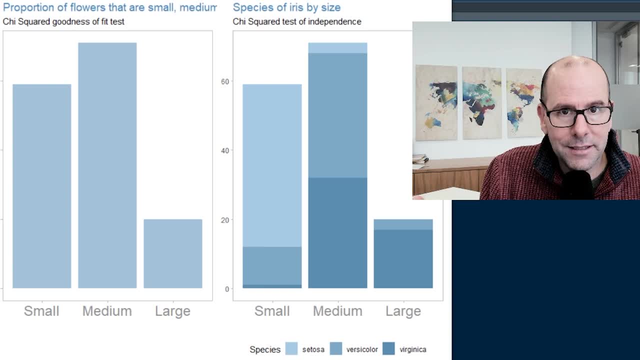 threshold we talked about usually 0.05, but it could be anything, depending on what it is that you're trying to measure and how important your sort of discrimination is. If that p-value is less than the threshold and we reject the null, we accept the alternative and we say that this. 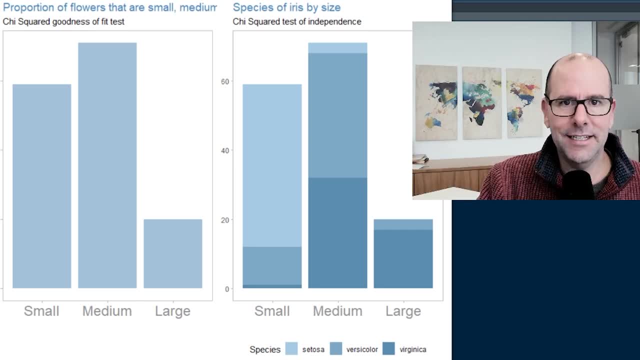 difference that we're seeing in the data is, in fact, statistically significant, And the exact same principle applies to the chi-square test of independence. We're asking the question: are the proportions of our species? are they in any way dependent or are they independent of the? 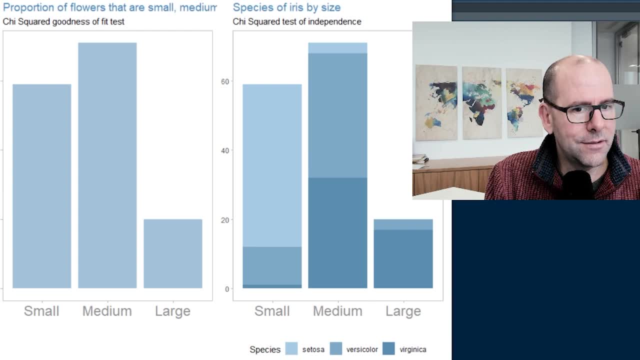 size of the flowers. Does knowing the size of the flower tell us anything about the probability of a particular flower being independent In one of these species? right, Looking at these graphs, it seems that that is the case, but we need to demonstrate that statistically. So we do a chi-square test of independence and we get a. 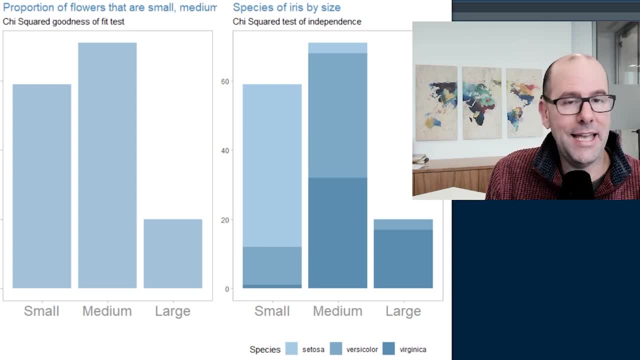 p-value. If the p-value is very, very small, beyond a predetermined threshold- remember it has to be predetermined. you can't do it retrospectively, that's p-hacking, bad science. If the p-value is very small, in other words, the probability of a sample showing a difference in proportions- 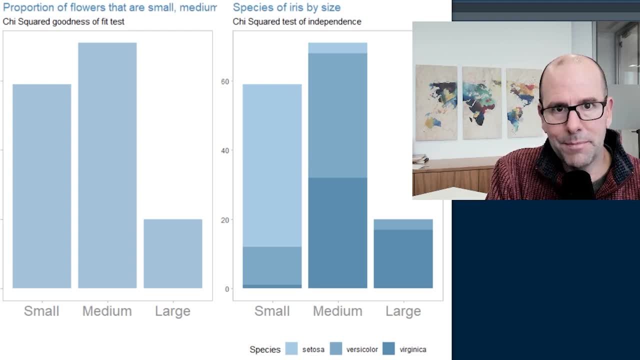 or a probability of a sample showing a difference in proportions. that's a p-value. If the p-value is a relationship which is demonstrated by a difference in proportions of this magnitude or more, the probability of that being the case in the event that the null hypothesis was true. 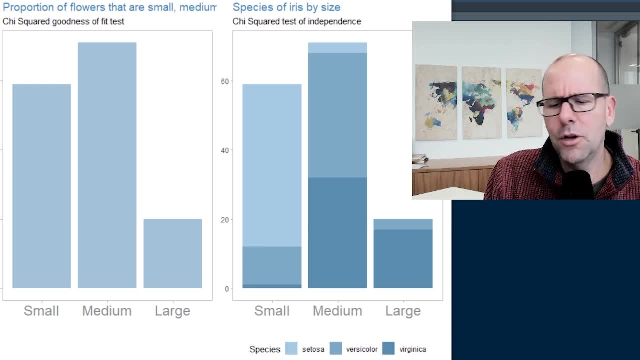 in other words, that there was no difference. if that probability is extremely small, we reject the notion that these things are all the same, that the proportions are the same, and accept the fact that, in fact, what we're seeing in the data, this difference that we're seeing, 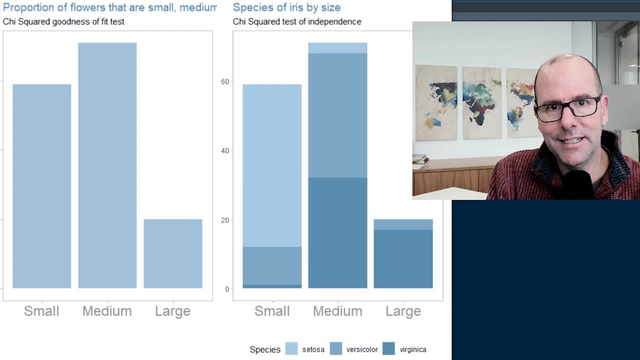 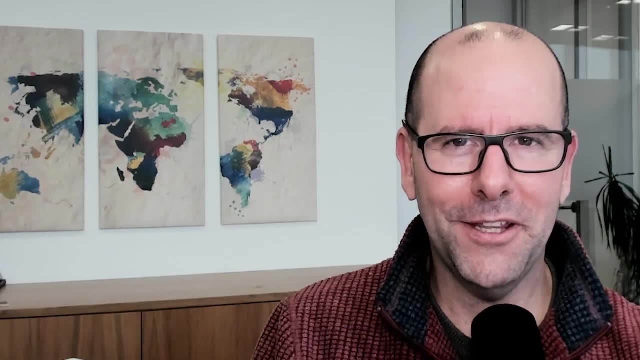 this relationship that we're seeing is, in fact, statistically significant. right, That's the chi-square test of independence. Now stay and watch another video. Share this video with people that you think might find it useful. Subscribe to this channel if you haven't Hit the bell. notification if you want notification. 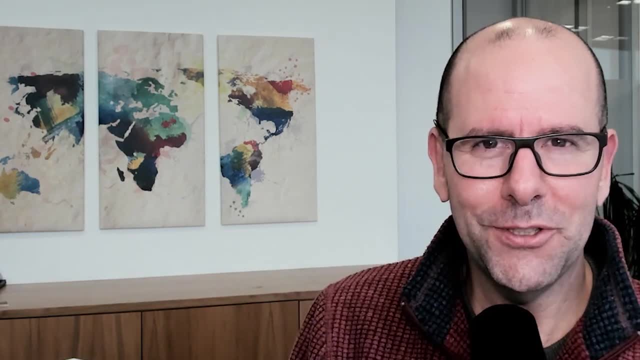 of future videos. Take care, Don't do drugs. Always do your best. Don't ever change. Speak to you again soon. All the best, Bye.